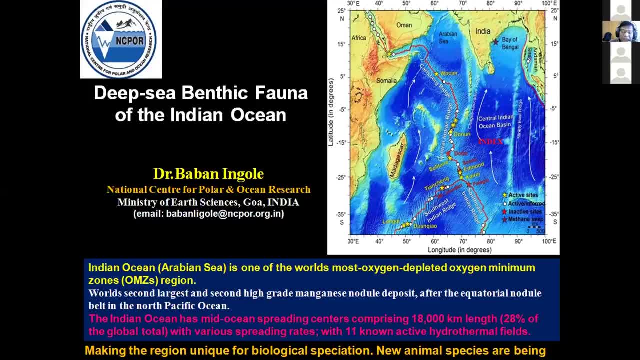 these are the unique with respect to the survival and also evolutionary perspective, and there are reports that on the regular basis, new species was being discovered from this area. When we talk about these resources, I would specifically thanks some of those you know, countries presently very active in the Indian Ocean for the deep sea. 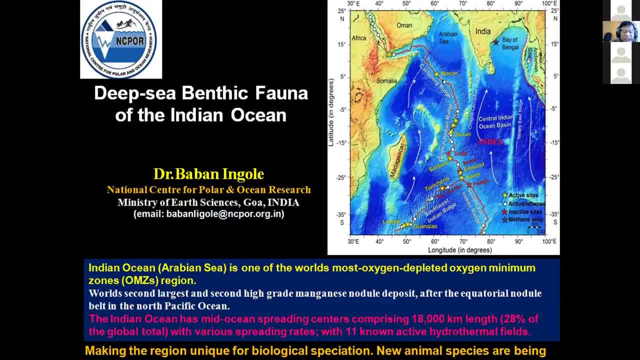 resource mapping and it is only because of this, some of the mineral resource, like the polymeric nodule or hydrothermal rain, or the- you know- sulfites and the cobalt crust, because almost 30 years back there were very few players other than India to invest in the deep sea. 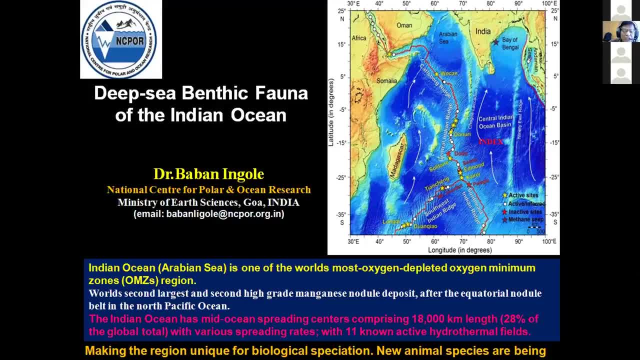 deep sea research in the indian ocean because there was no specific attraction. deep sea study itself is a very expensive affair and unless you have some attraction nobody will put up the money there because you don't know. it is a blind game. but for last almost two decade many countries are. 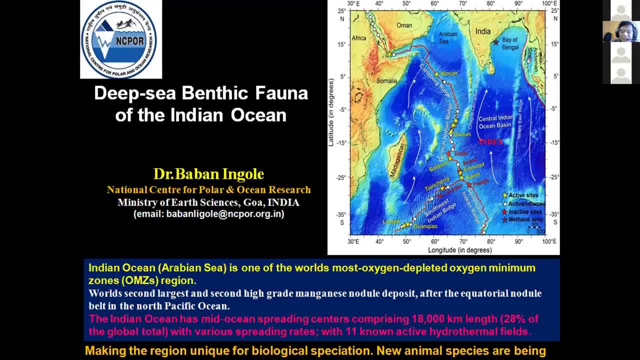 coming forward and doing the research in the indian ocean and contributing a lot to the science and specifically it is as i can, you know, see some of those countries which are investigating. looking from the future, you know benefits whether it will come or not. time will prove that, but presently it. 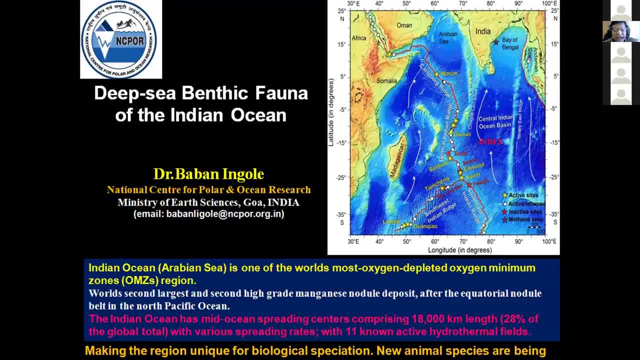 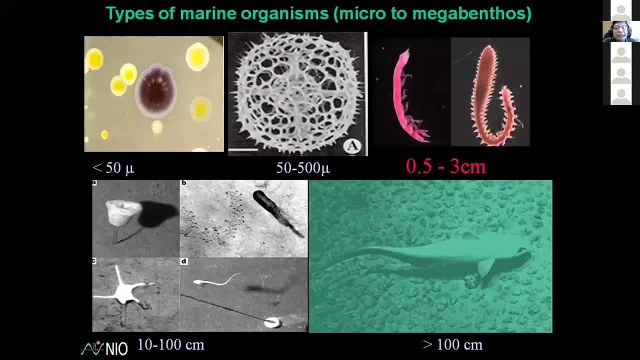 is helping the science and i am for that. you know, as far as getting new data, we required somebody to to fund those research programs and that's how it is happening. so with this introduction, i am specifically going to talk about the deep sea macro fauna- myofauna, megafauna- but specifically 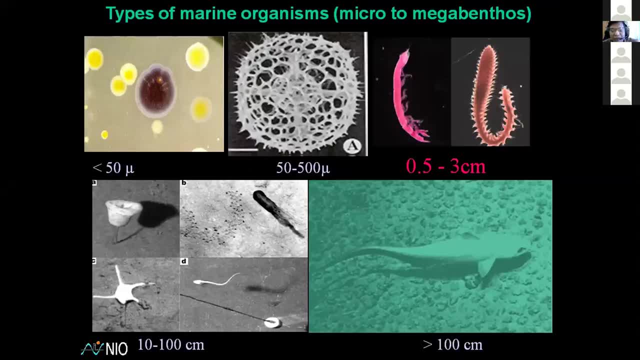 we'll talk more on the macro fauna and most of you are aware about it. i have just, you know, put up some pictures just to see about the size fractions and just to understand. we have the bacteria or bacterial size forms. we have some forams and myofauna, then we have. so this is micro fauna. we. 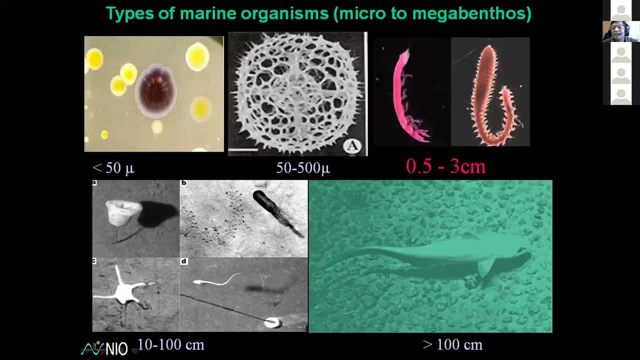 say, or micro benthas, these are myobenthas and these are the 0.5 to 3 centimeter. what we have about macro benthas, and bigger than all these things are the mega bentha. so this is how the classification, you know: classical, traditional. 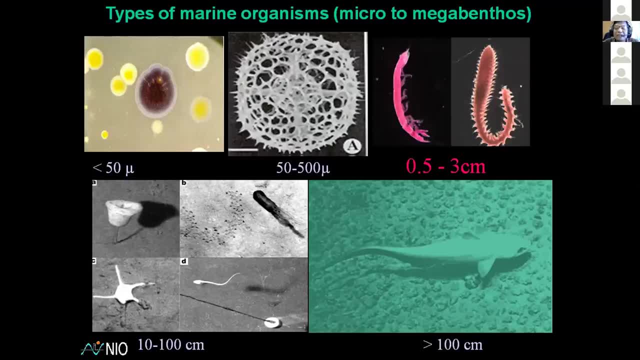 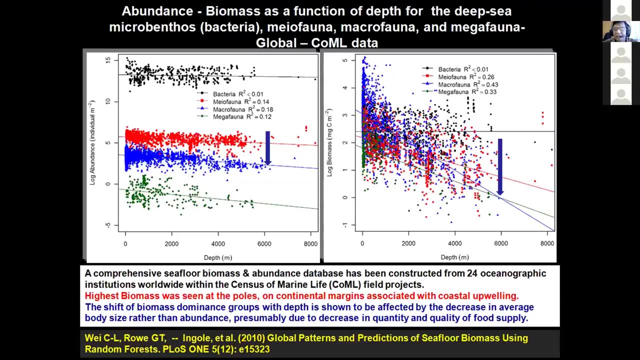 classification of benthos is, you know, followed by the benthic ecologist. when we look at it, you know we did during the census of marine life program where mark was, you know, very active and coordinating many programs. we worked together during that time. this is the product of census of marine life where we have worked. looked at the deep sea, benthos. 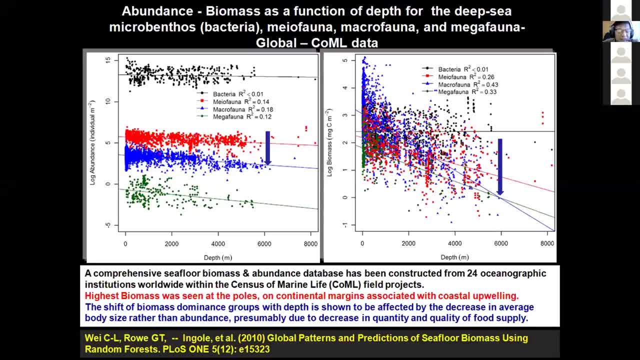 a different fraction, and all the data were synthesized together with, you know, gilbert row and his student work together. we all have supported them with the data and the exercise is, you know, put up into these two graphs, as you can see that there is a, you know, abundance and 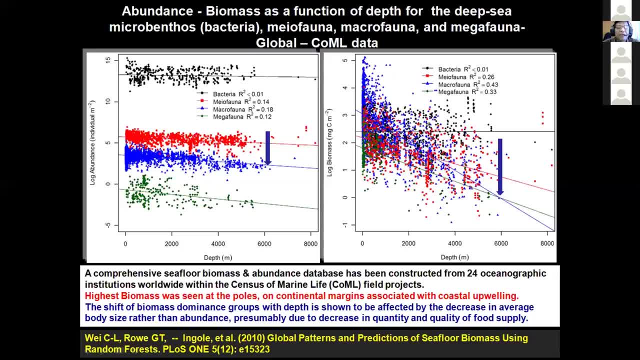 biomass and fractions. you have bacteria, myofauna, macrofauna and mega. as you can see it, you know there is a difference in the pattern if you look at it, and the pattern is importantly, if you see it, the abundance in the form of, you know, shallow water to deeper water and if you look at it, the 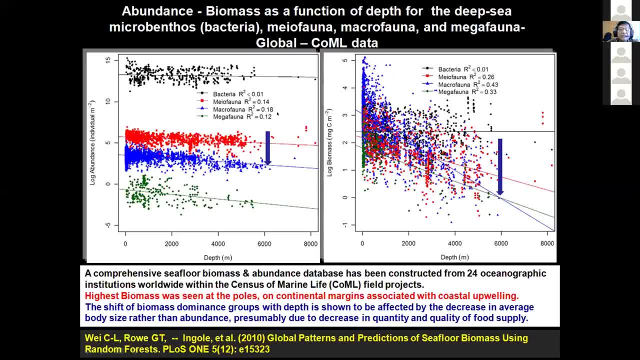 bacteria. as you can see it, this myofauna, macrofauna and megafauna megafauna- you have got a large size and therefore individuals are very high in the, you know, shallow water and this is obviously because you have got more food available in this area, although you know the 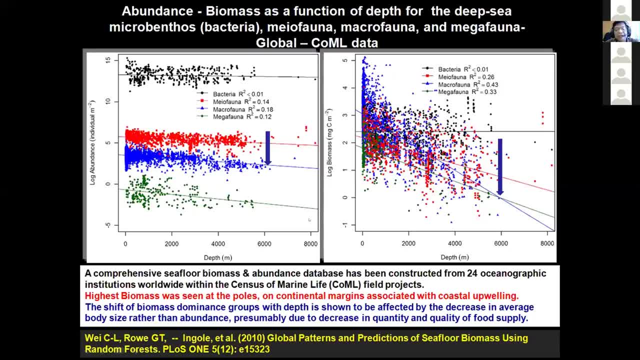 here will be: the abundance will be very high initial. as you go deeper, the abundance is reduced drastically. with, with you know, are much lower and the Myofauna produce阿nd is very high and they previously had one thing that was, which was somewhat opposite, but this, at least on average, has given an 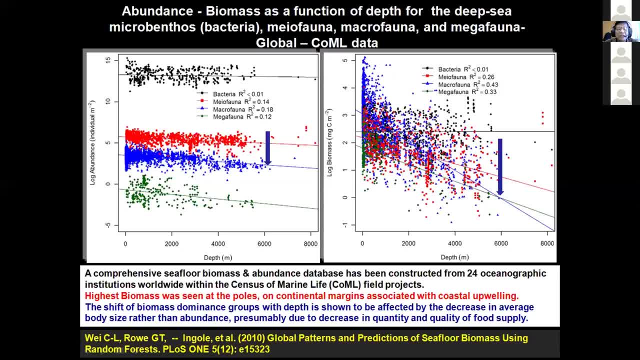 increased here that the left is 7- 2016, которой in the deeper water, but not like what is in case of macro or megaphone. and if you look at the second graph here is, you know, different picture altogether in terms of biomass. biomass changes very fast. 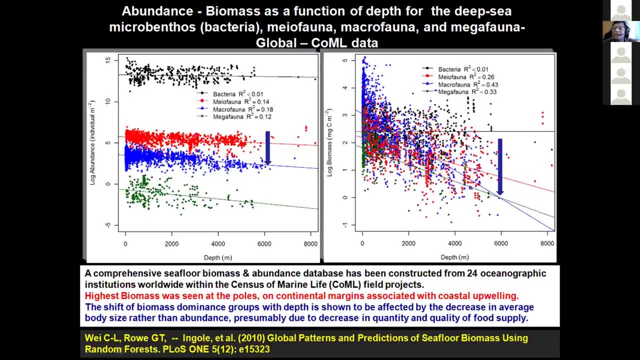 with respect to the depth changes in the deeper water, but again, again, more so in terms of megafauna and macrofauna, but not for the meophauna. so meophauna is one which sustain the stress of depth and resource crunch and therefore they're very interesting to study. 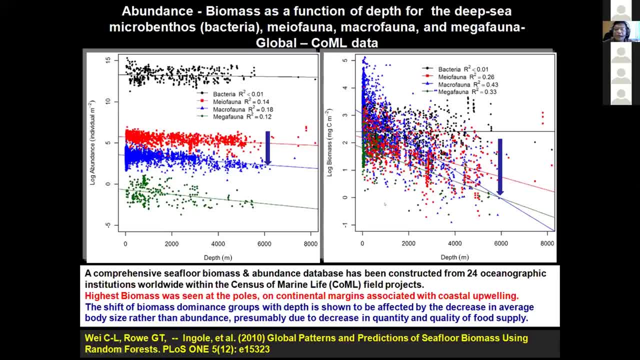 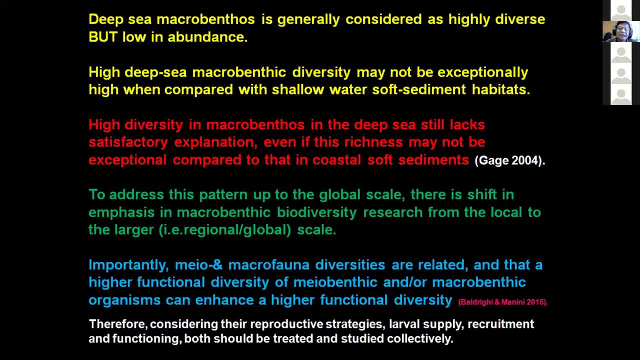 in terms of their ability to use the resources both in shallow and deeper water. so this is how it was put up in the: a global picture. we know what we consider. you know usually that you know deep sea microbials, generally considered to be highly diverse but low in abundance, as i already mentioned it here. 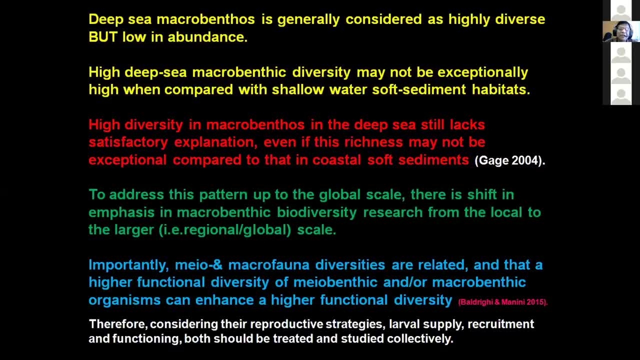 then macrobe diversity may not be exceptionally high, but compared to the shallow water, but it is, you know, certainly high in the abyssal, plain and shallow sediment. as far as the diversity of megafauna is concerned, it appears to be. appears to be, it is not? it concluded as i 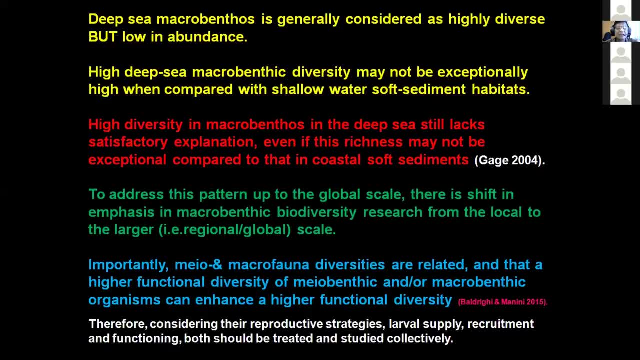 understand, appears to be high in the rich region or seamount region because they're specific to that compared to the other areas, and this couldthis could be because of the reality of, uh, the words the did you know about, at least you confuse a lot of things, whether it is web nose, medium vault orрахin conversation. so when the mechanical 하는, then 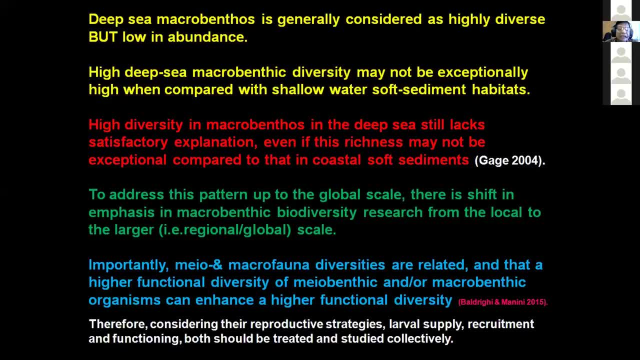 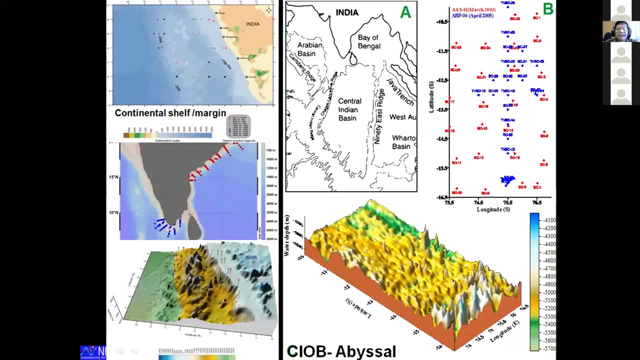 hareung region, because the specific to that compared to the other areas, and this could be because of the compared to the other areas, and this could be because of the resource availability. What we have done, it, you know, last almost two or three decades we have sampled Indian. 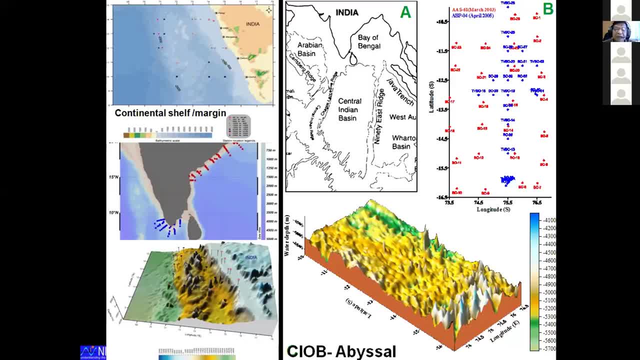 ocean in different parts, for example shallow and coastal waters, both in Arabian Sea and Bay of Bengal, like here is the Arabian Sea from the shallow, almost 20 meter to 3500 meters, both Bay of Bengal simultaneously, also some specific area in detail, then the deep sea. 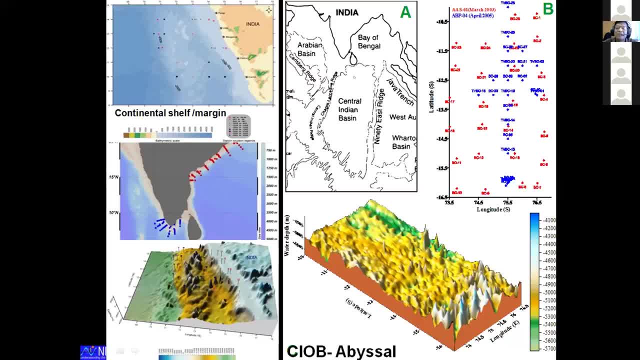 particularly interest. our interest earlier was central Indian basin. we all know that it is the rich area for the- you know, Nodal deposit and future prospects are there for mining prospect then, along the ridges we are. presently we are working under the India's deep sea mission program on along 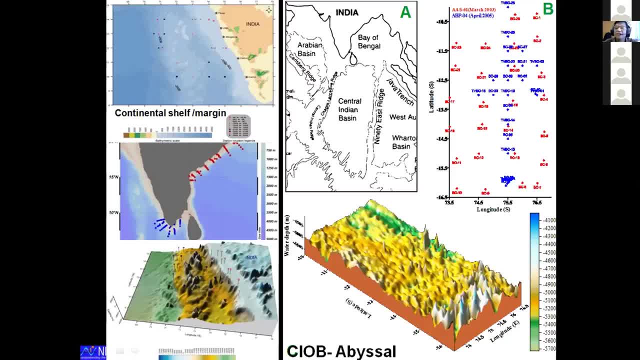 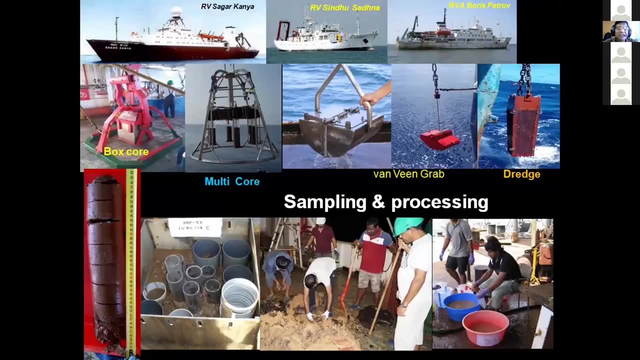 the ridges and as well as the you know. So these are some of the station locations where we have sampled, in the Shelf region, as well as in the Abyssal region, and these are some of the you know equipments, what we have been, you know, conventionally used. 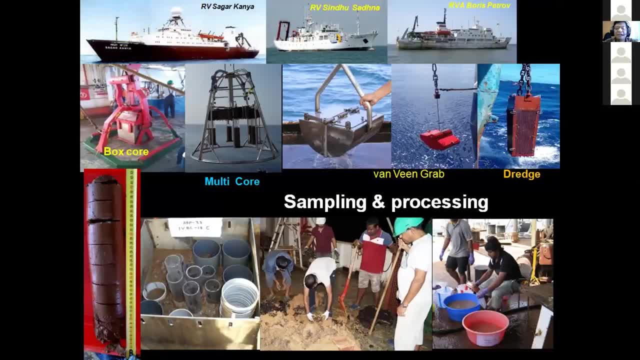 We have been using for the deep sea sampling, like initially, we are using, you know, Van Wyn grab or Peterson grab came to the you know most precise box corer. then we are now using, for last couple of years, the multi-core. then also we are using the benthic sledge or you. 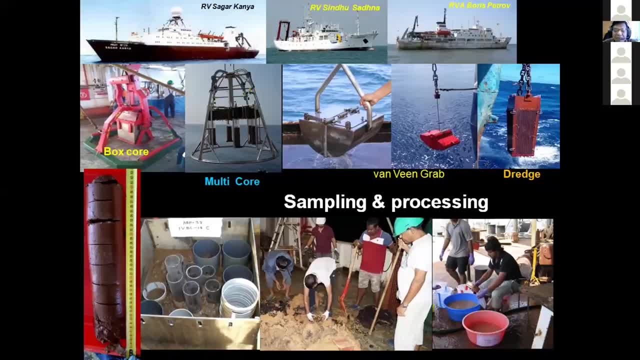 know, modified dredge for the- you know megafauna sampling and the using the standard dredge for the deep sea sampling. So we have been using for the deep sea sampling, like initially, we have been using, you know, standard techniques. the samples are, you know, processed. most of the time we have used 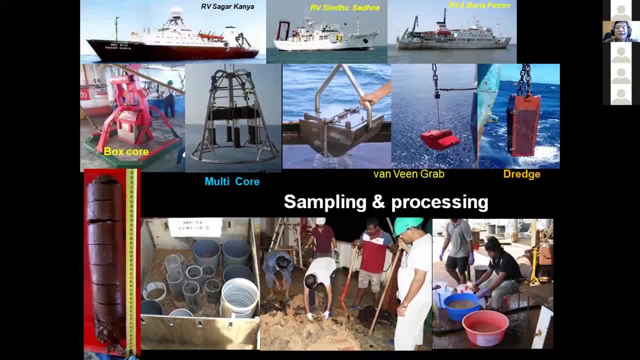 you know, the research vessels belong to ministry of public sciences or the CSR national institute of oceanography or sometimes even the higher. you know, charter research vessels are used for collecting the samples and we collect, as I told you that you know, bulk samples with the box corer or the Van Wyn Peterson grab or sometimes with the, you know, multi-core. 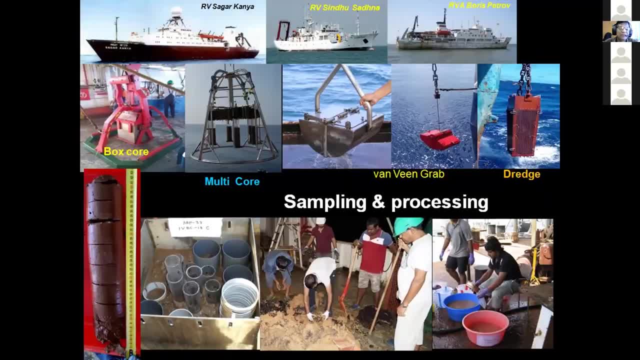 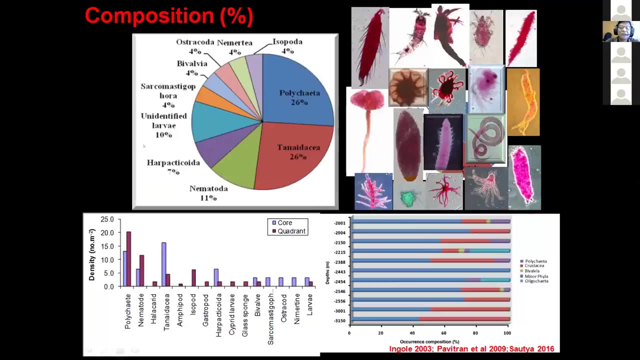 or the University of Vancouver to get a better understanding of the information that we have collected. So those are the techniques we have used for the deep sea sampling. then you may also use- you know- heterogeneous samples, as you know the. you know the different types of samples you have used. 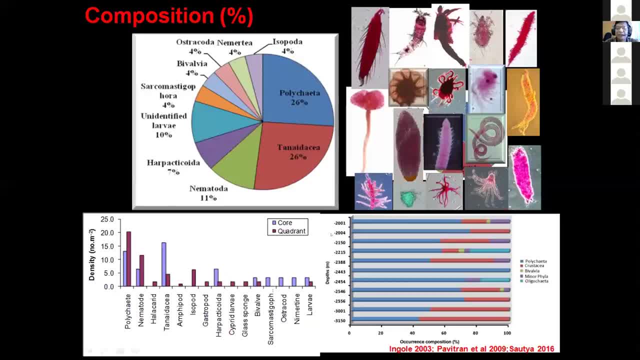 OK, Will tell the next result. I'm showing it here. We do have the species composition also done. These are some of the major representative of the group wise, as you can see that Most of these are also coming. you know temporary macro fauna, because they are permanent- myofona, small size like copepods, and 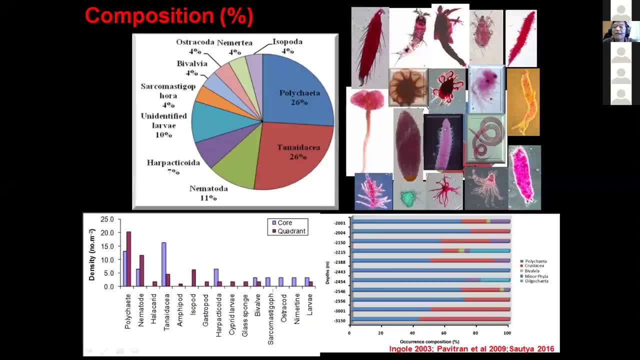 nematodes, but then there are polychaetes and other organisms. we have permanent macro fauna. So what has been recommended in the deep sea studies is that go for the finer size so that you will not miss those fine fractions of the fauna. and therefore, if you use 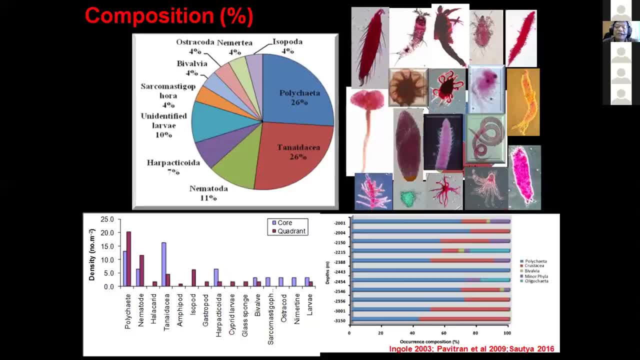 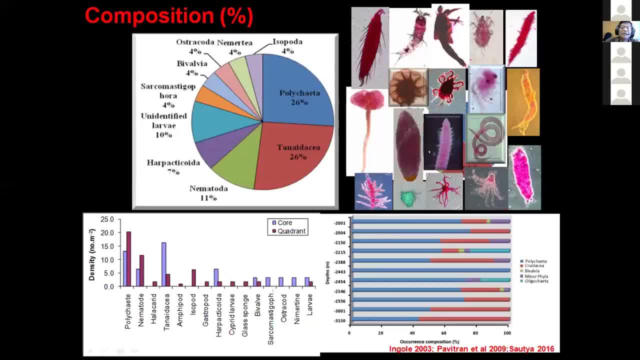 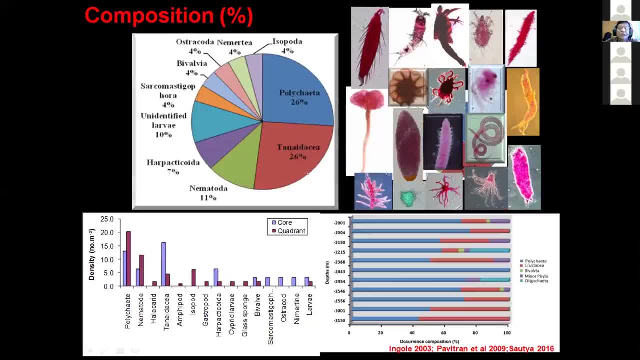 myofona. So these are the dominant group. as you can see that in most of the macro fauna- Sub-sediment macro fauna- you'll get polychaetes and crustaceans are the most dominant and crustaceans it will sometimes polychaete will be the most of the time the dominant one, crustaceans sometimes you. 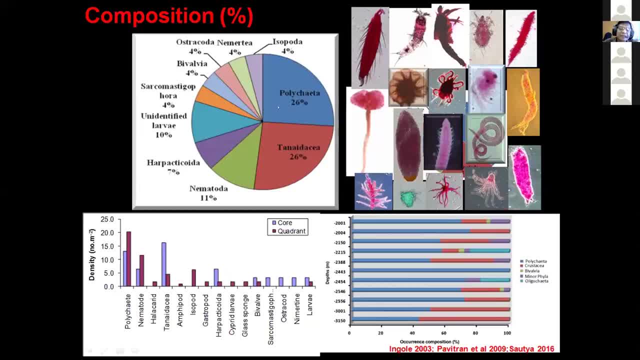 might get isopore mp4 or tannates here. in the case we had, tannates were there, isopore mp4s were there, but not that. we do get a large size myofona, more than one millimeter, and therefore it is retained. 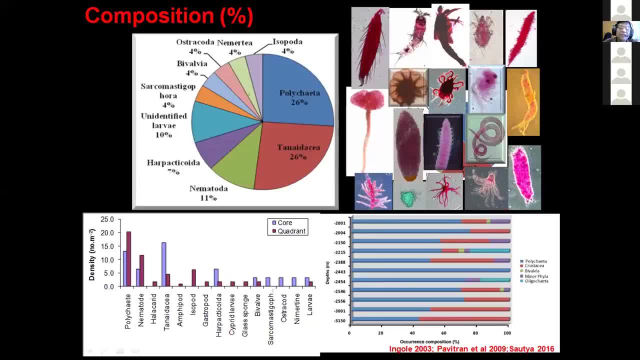 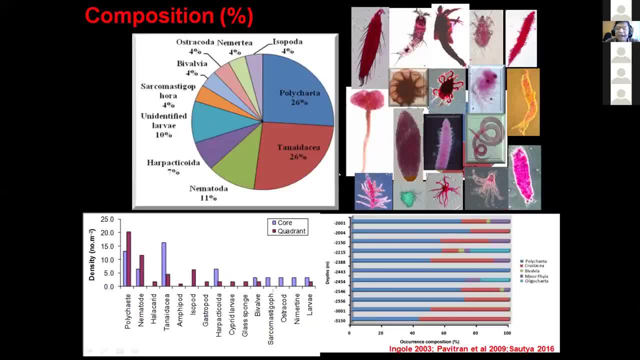 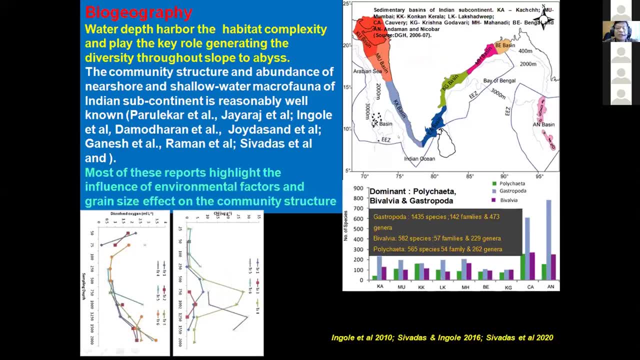 The micro fauna we were talking about. this is meofona. it is a micro fauna, That's the meofona in the micro fauna, but we have specifically mentioned it very clearly that these are the temporary macro fauna and this is what it is. as far as the coastal studies are concerned, we have 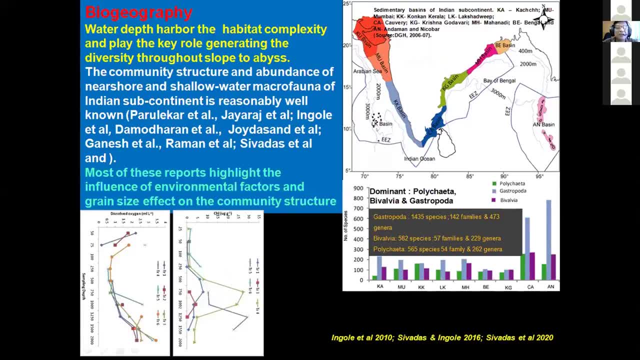 sample, as I told you that, both east and west coast very meticulously over 30- 35 years, and there are different groups of work. I'm very happy to share that there are more than 10 phd studies, NIO as well as Cochin University, and some of those people are doing very well such 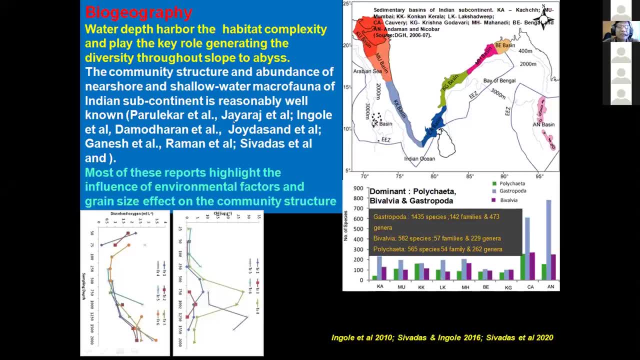 as the Jaradas Jaras who have worked with Dr Damodaran. then there is Ganeshan, who worked with Dr Raman, Shivdas Sanitha, Shivdas Sabyasachi Sautya. these are the work with 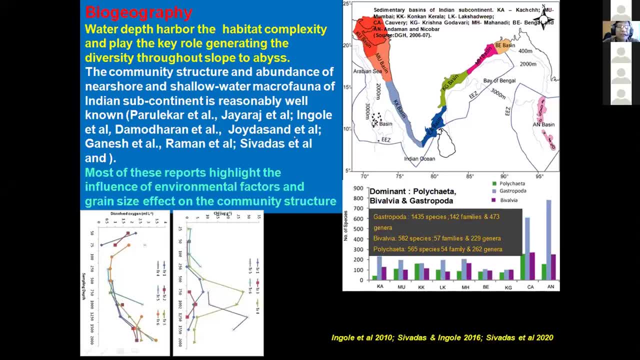 NIO and they are active. you know I can say third generation benthic ecologists. you know we are working quite well and have come up with very good publications and those when we synthesize- Sanitha Shivdas and myself, we have synthesized the data, the quoted Indian. 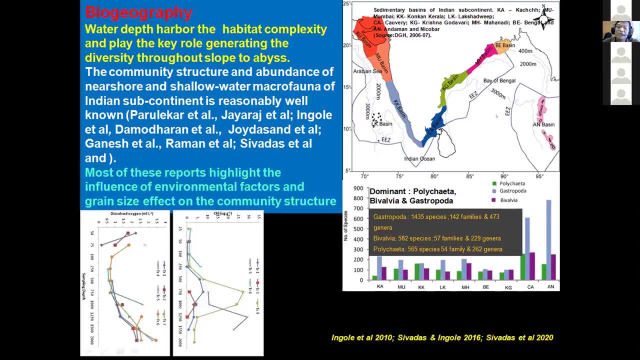 data and we could see that, both east and west coast, there are typical groups representing each benthic ecologist And these are the sedimentary basins. what we have, you know, divided based on the sediment characteristics. for example, on west coast, we have, you know, Kutch, or you know. then, 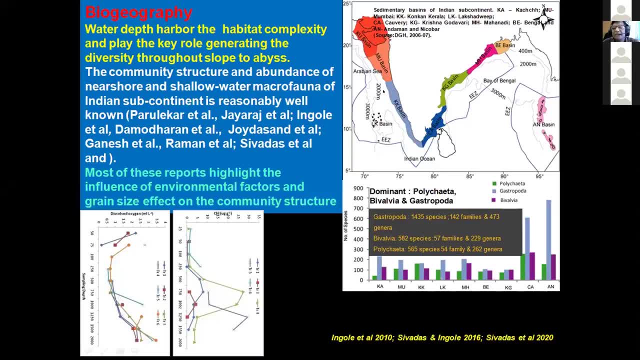 Kutch, Mumbai basin, then you have Kaukan basin, then you do have it, you know Kaveri basin, KG basin, which are well known commercially also as far as the you know oil and natural gas is concerned. and then you do have it, you know Manadik. 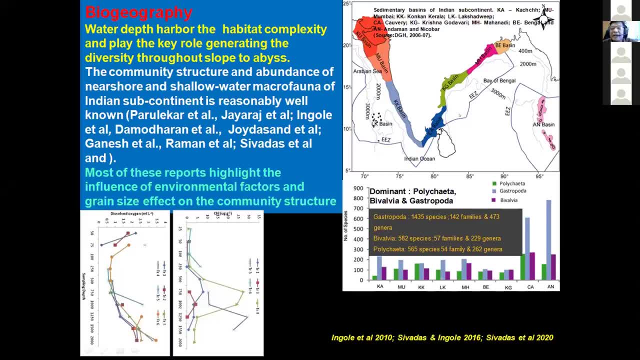 These are sedimentary basins, depending on the fact and also the composition of these forms, specifically the macro funnel composition of this, The dominant group in this particular exercise. we have seen it where the polychaetes and bivalves and gastropods 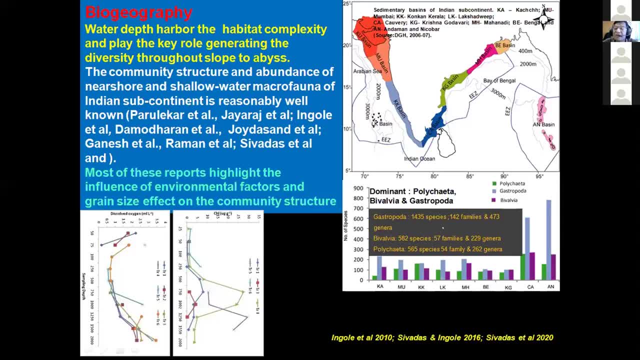 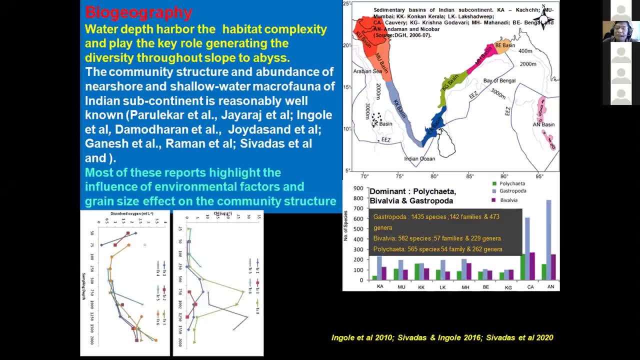 in the you know, in the you know in the last you know session for over 400 gender and these are most of the data is from the OBs. so it is data is curated. we can definitely see because either this one PhD, this is all the published papers, and so georeferencing. 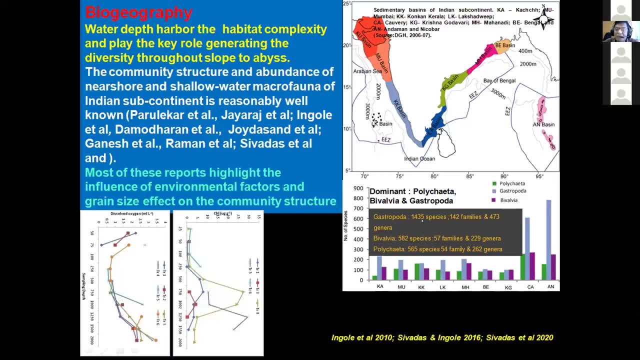 for all the data was checked and found and therefore bivalves, we had around 582 species could be. figure could be more, because this is published in 2016.. So, polychaetes, as I was just telling you know. 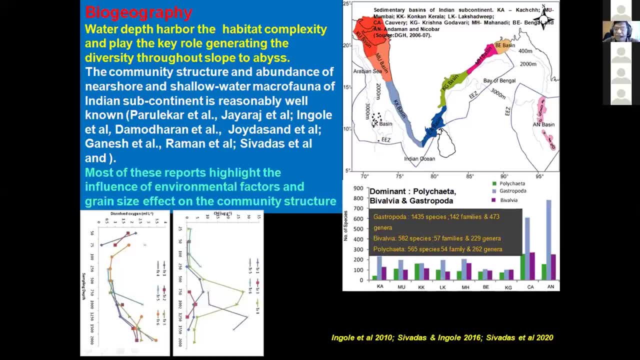 … one of the dominant group, or 565 species are reported in along the both india east and west coast. so there are three most dominant group: we have polykids, bivalves and gastropod. in terms of the speciation, as far as the resources are there, as, as i was telling that arabian sea is one of the 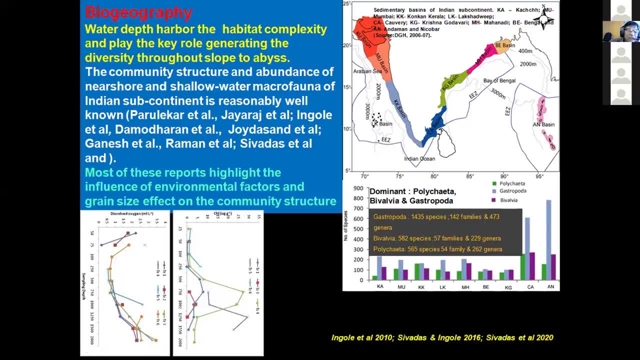 you know, largest omc area and therefore oxygen is the limiting factor. then the food, as far as the deep sea forms are, there certainly is both in the form of shallow water. you have the chlorophyll, you know flux coming from the surface. also there are, you know, seasonal fluxes. so we do have it as 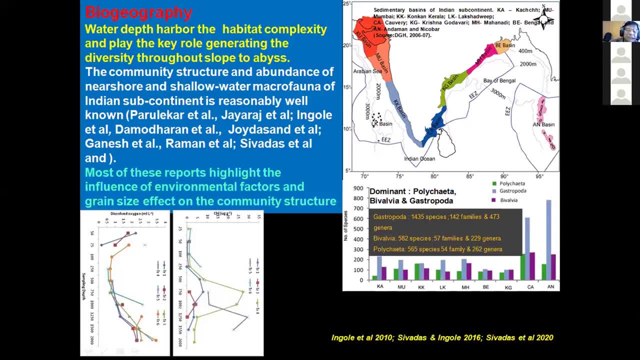 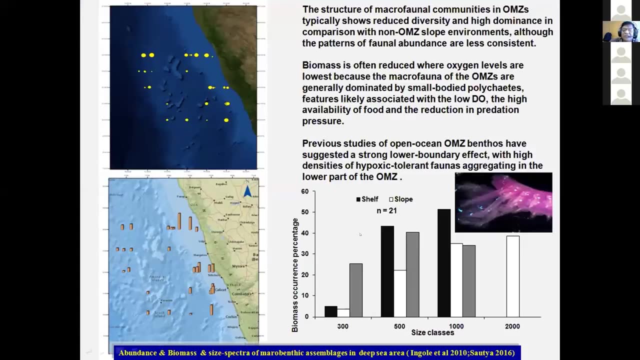 you can see that in this graph, you do get the chlorophyll, even in the deeper water and dissolve oxygen, as, as you can see, the depth wise profile in the arabian sea and are shown it in this one. well, uh, if you can see it in this graph, we have the structures of size fraction. we have, you know, seen. 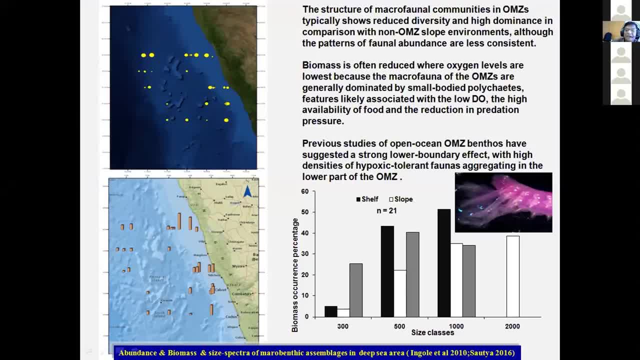 it both in shallow and deeper waters, and here you can see that you have a larger forms. you know, particularly percentage of the larger or mid-sized forms was in the mid-depth between 500 and the thousand five hundred meter water depth. you do have a smaller fraction in the mid-difference. 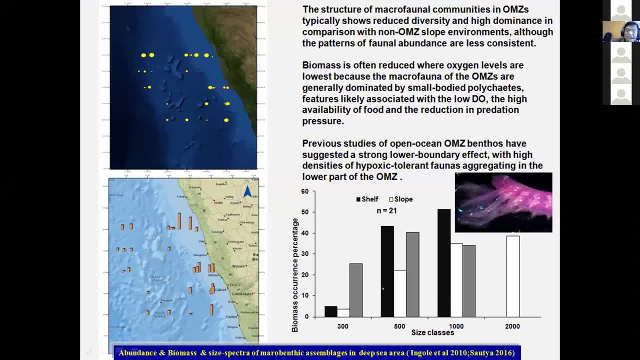 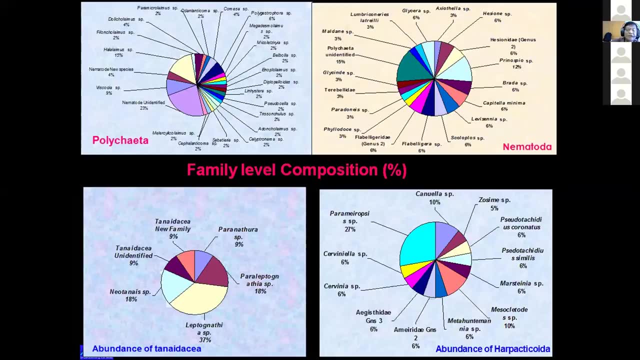 in shallow water as well as in deeper water. so this is the one which you know, mostly in the slope region itself and slope region you have got, you know, medium or average size macrobenic species. you do get it. uh, if you look at it, the species, or you know not all the species. 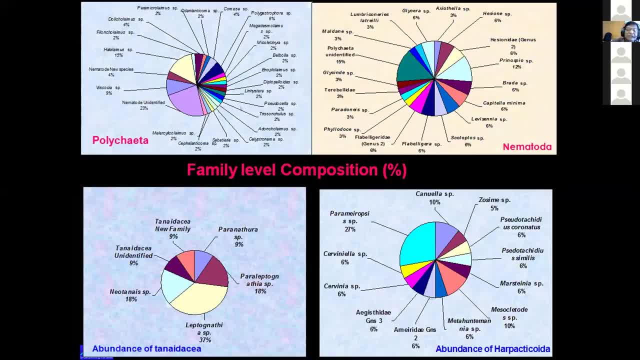 are identified because, as i, as i was telling that the this is like ongoing studies are there and, as an example, you can see the social species that we have. also, we have thisucking ecosystem in Bahrain and then you get, like the ussari species, but more in this view this year. 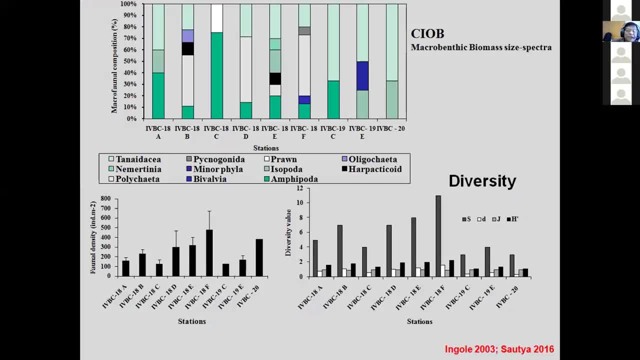 neofuna and we have got that also very well. this is: we try to see how diverse these forms are there with respect to the specific site locations which we have been sampling in central indian base basin regularly for last almost 30 years, and when we say seasonal variation when we visit it on. 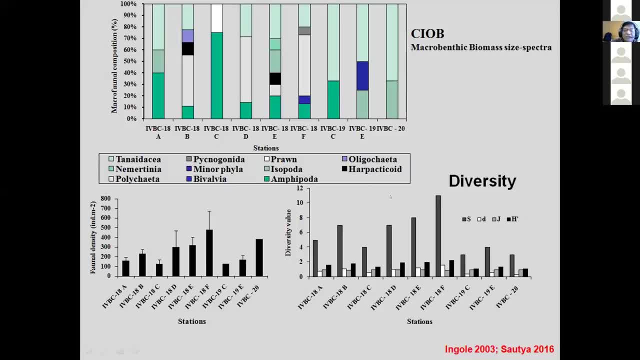 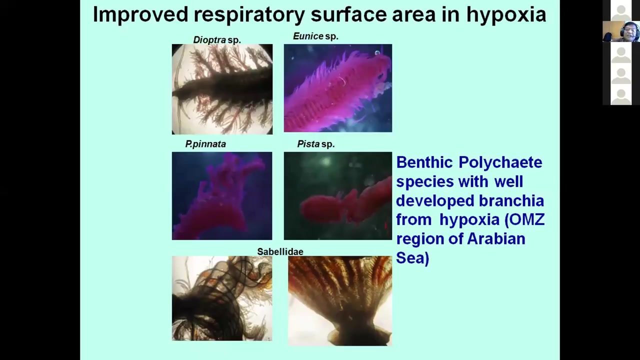 yearly basis there is not much variation as far as the abundance is concerned. but biomass we have seen there is a variation and it could be largely because of the availability of the food resources in the regions. there are some species, particularly in the in the stress areas and in the oxygen minimum zone. what we have seen so opposite condition in 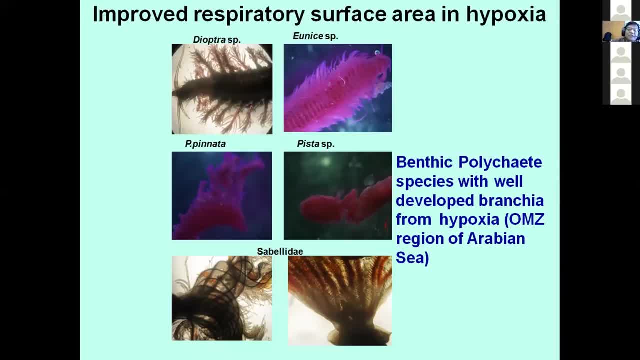 the in the stress areas there are, you know, for example, polychaete species. one of the most dominant was the a parapinus pinnata, but we do have it. other species present there and specific adaptations of these species to the low oxygen conditions are. they enlarge their branchias to, probably to store. 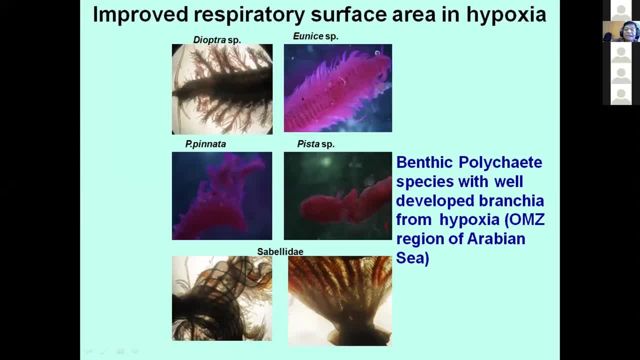 the oxygen when there is a- you know- high oxygen present in the area and then afterward use that is a low oxygen condition. that's how they adapted to the conditions and survive when other species cannot survive. they have the rich food resources, but oxygen is very low and therefore they utilize. 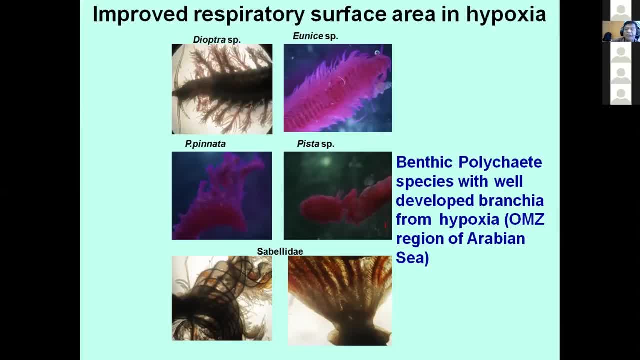 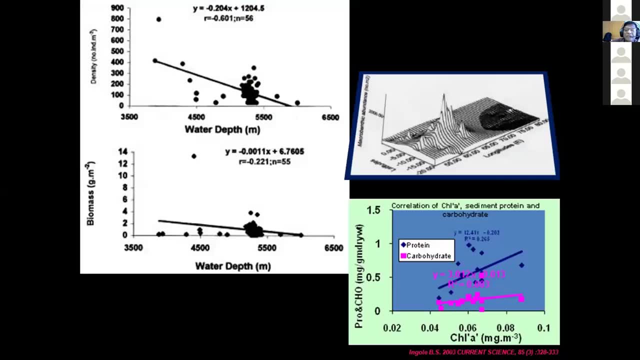 that conditions and proliferate for their self. you know, population increase or prolification. so these are some of the adaptations, these, these species do have it. what we have i, i just mentioned it, you know, in the first slide for the global picture, as you can see, for the central indian. 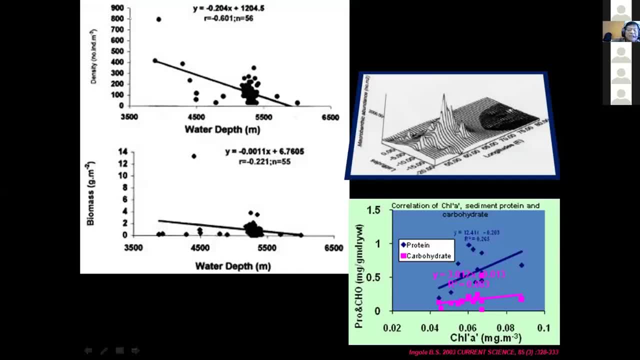 basin, both in terms of density and biomass, and this is how it changes with respect to the you know depth. so we have 3000 meter, mostly the deeper water i'm talking about, because that's the depth. we get it when you go deeper waters, more than three thousand to six thousand five hundred. 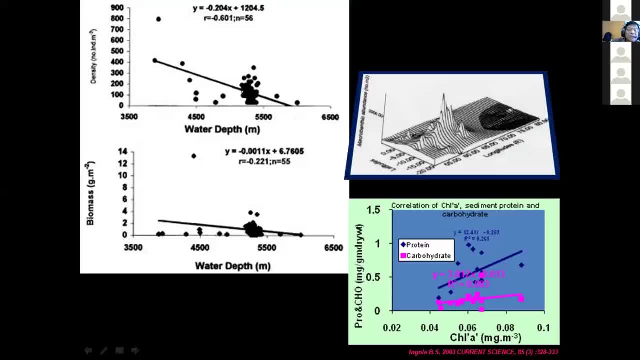 meter and we have the density of macrobenthos per meter square and here's the biomass, you know gram per meter square and as you can see that you know we do have it around the you know 5000 meter where we have quite good observation, because these are the areas where our more. 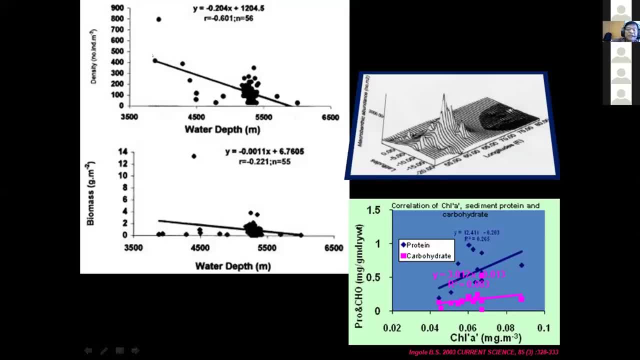 sampling has been done, but otherwise, if you can see that as resources get limited, the density and biomass also reduces. that's why, but you do have some patches and this is where you can see it. we have the- you know, uh, abundance of macrophona here and here. longitude, your latitude. 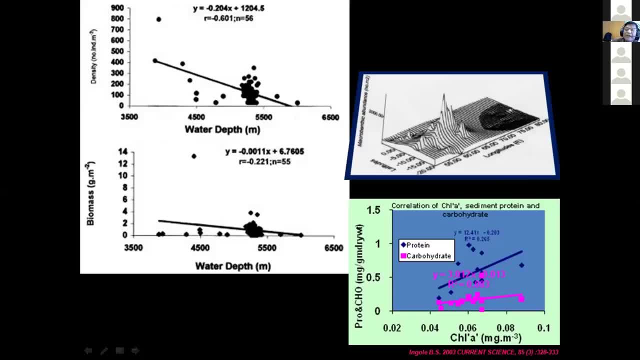 and there are some patches where you do have it very high abundances, uh in the central indian basin. now what is important here is the your you know food, and here we have got the you know uh carbon, and here is the you know elohim concentration, so chlorophyll and uh elohim. 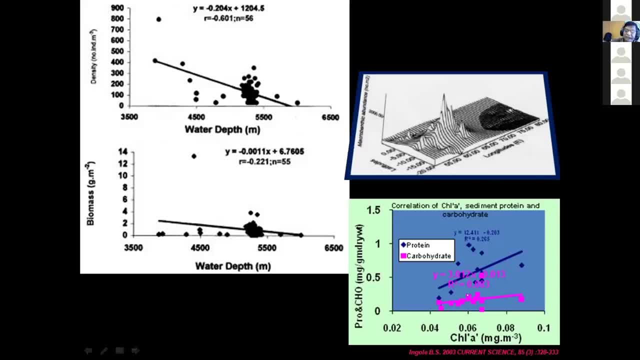 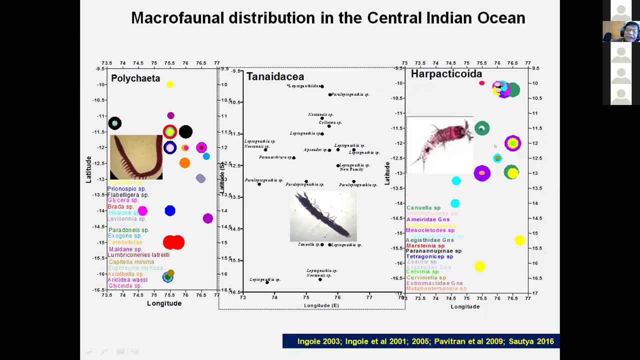 concentration? how do they match it? so seasonally available flux is the major food for the deep sea life in this area, so that signality is very, you know, clear in some of the both shelf and slope area. that's what we have concluded is. i was just talking about the difference. 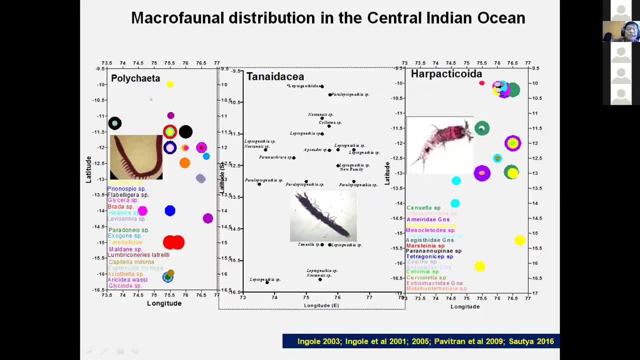 you know, species, uh, what we have seen, and the distribution, uh, in the deep sea, particularly in the central indian ocean, as you can see that, from the 10 degrees south to the 16, 17 degrees south, we have sampled repetitively in this area. and here are the distribution, our biosphere. 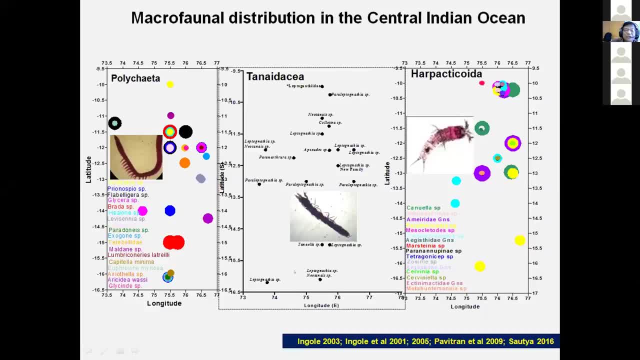 distribution. some of the species of polykits are shown it here, candidates distribution is shown it here and herpacticoid copepose are shown it here. so there are the patches, as i was telling you that very high diversity in some of the areas. this one reason i could say that why we have got high diversity in this region is 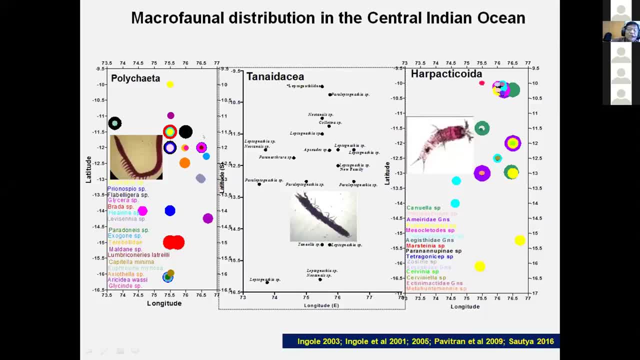 we have more samples in this region, so we can't say that this is only the high diversity zone. you do require more sampling in some of other areas to make it the you know conclusion that these are the only areas where you have high diversity. this could be the sampling. 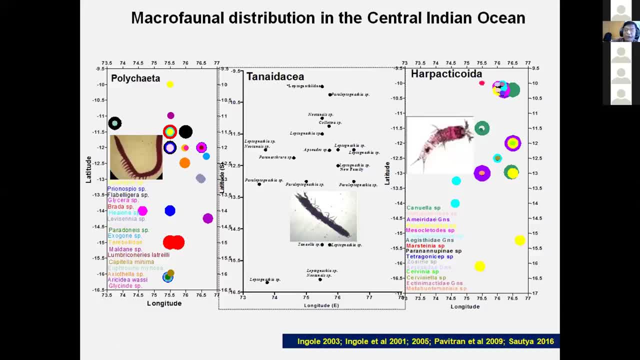 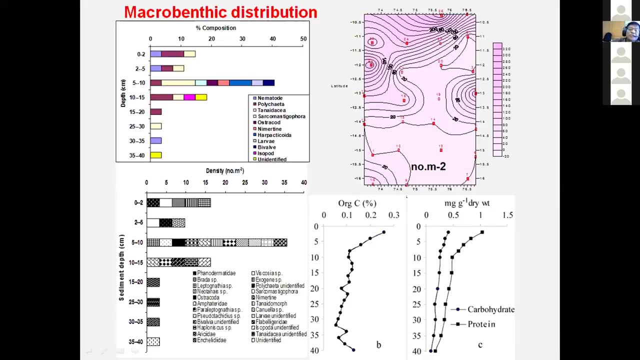 you know bias, because we could sample more, we have got more species, which is also known that in deep sea if you get more sample, it tend to have or result into the more species. as far as the surface distribution or the horizontal distribution, i showed it in previous slide here at 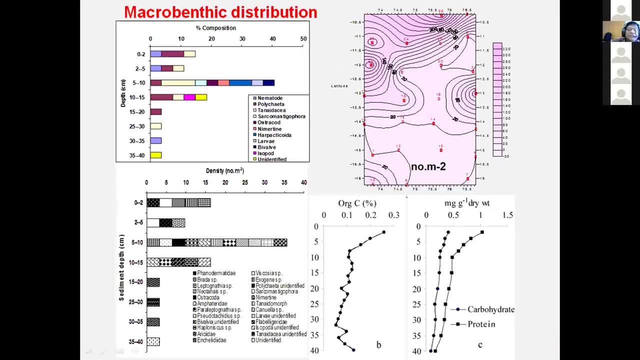 some of the sites where we have repeated sampling, we also have a more quality sampling distribution, have seen the vertical distribution of benthos, particularly macro benthos, in the sediment, and it was specifically for the purpose, as i told in the beginning. only this was part of the our 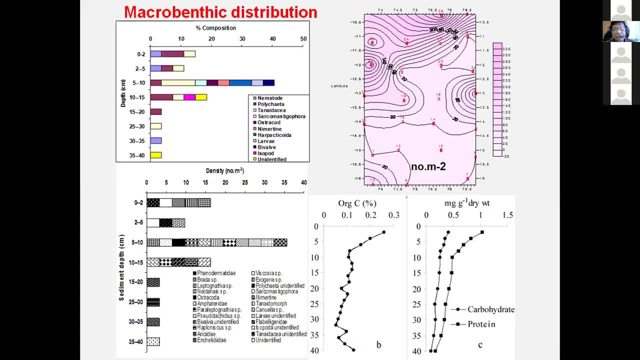 environmental study for the polybrytalic nodule future mining program and therefore we wanted to also see that if nodules are available vertically in the sediment, how deep they are and what type of life is associated with that if it is there and therefore the vertical distribution we have. 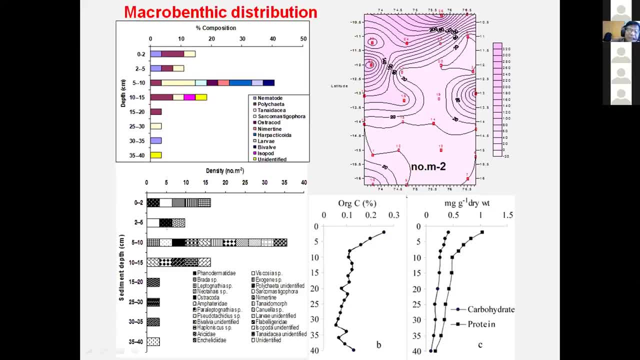 studied up to 50 centimeter. samples were taken. even deeper also, we are taken, but we have seen it, the fauna present up to 40 centimeter. maybe you know the fraction of that percentage may be very low, maybe five to less than ten percent below 10 to 15 centimeter. however, it is present in that. 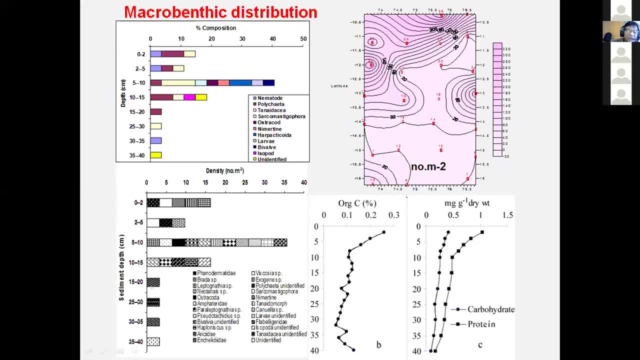 area, as you can see that, particularly from this graph, you have got five, five, five, so around you know, twenty percent. it comes below twenty or fifteen centimeter, whereas eighty percent is above and particularly top ten centimeter. you have got almost seventy to eighty percent of the. 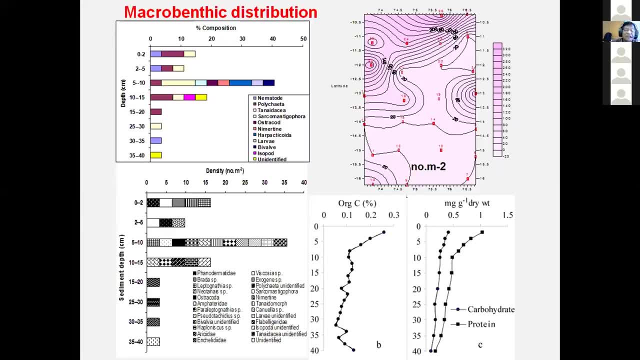 phenomena. so the top ten centimeter sediment layer is active. as far as the benthic activity is concerned, and that is the most important from the biodiversity point of view and that should be considered for more- you know detailed study, because if you take deeper sediment core, it is. 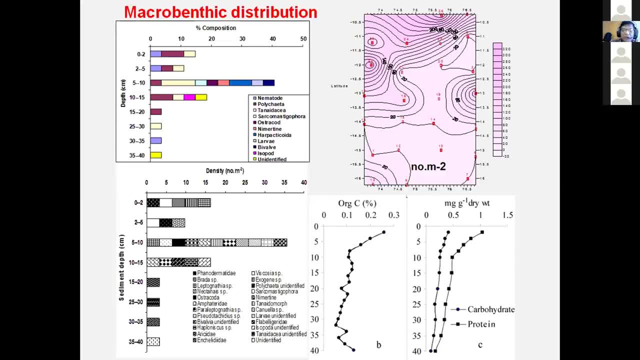 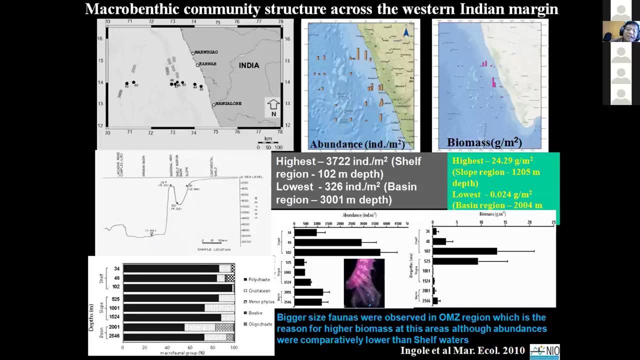 a time consuming and you will not yield more more than ten percent of the what you get it in the surface, five to ten centimeters. well, i already mentioned you that we also work in the shelf and slope region and the deep sea region, both east and west coast, and there are some results we you know. i have tried to put it just. 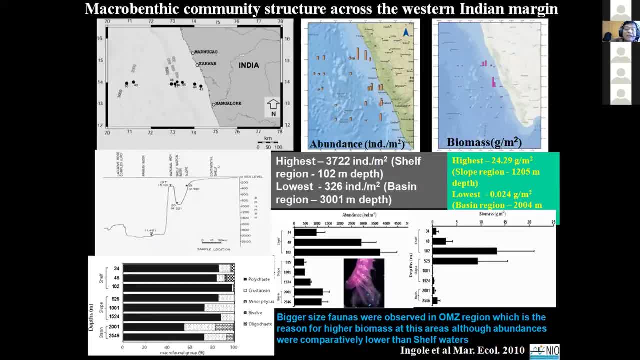 for the you know example here we took a two transect uh, one was of uh, between karwar and mengalore and one was, you know, of lagiri, and there were more transects. this was in detail. we have taken it from shallow to deeper water and went from 43 meter water depth to 3500 meter water depth. and what we have seen it that 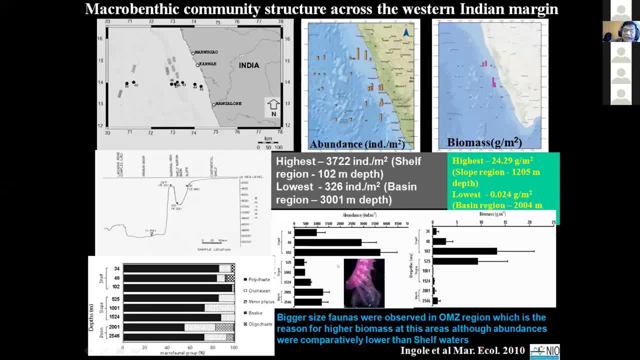 it was across the oxygen minimum zone area. so we do have itself, region representing slope, region and basin representing all the three. what habitat you get? it along the west coast of india and, as you can see that the depth between 500 meter and 1500 meter was the oxygen minimum zone and in that area, 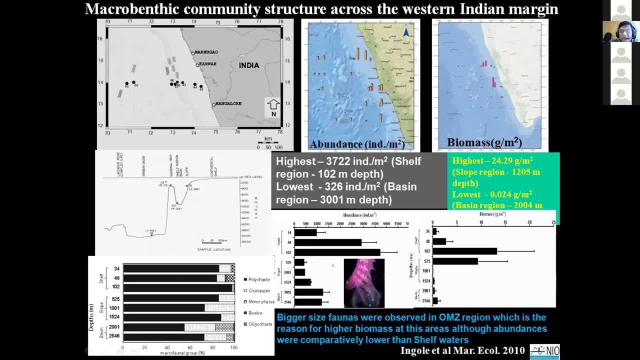 we do have it comes in the slow pleasure and we do have it. very low abundance in this area, high abundance in the shallow and then also in the deeper water and, as you can see that biomass was the maximum in the shallower zone less than 500 meter, very low. 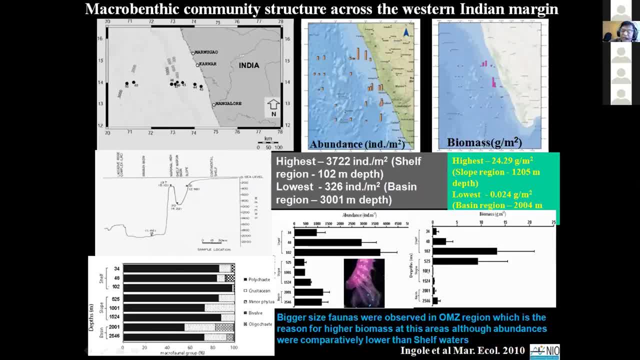 um is in the um is in the om is in the om Z area or oxygen minimum zone area, and then there is a little bit increase in the deeper waters. Now if you look at the representation of the fauna or composition of the fauna across the- you know water depth- you can see polychaetes are the most dominant, followed by the crustaceans. 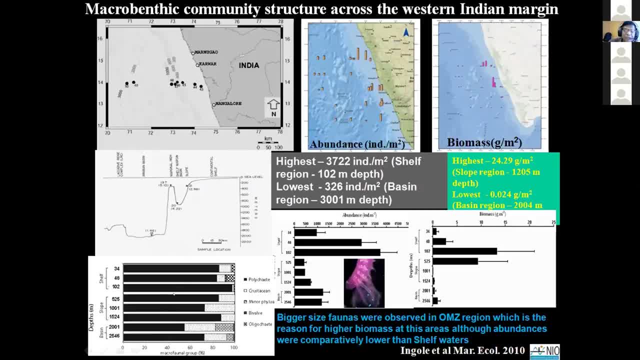 and that's what you know. then there are other forms, but most dominant are polychaetes, almost 80 percent, and then crustaceans, mostly isopod and pepod and tannids. depending upon the location it will be 5 to 10 percent, almost 80 percent the polychaete. so highest abundance around 3700. 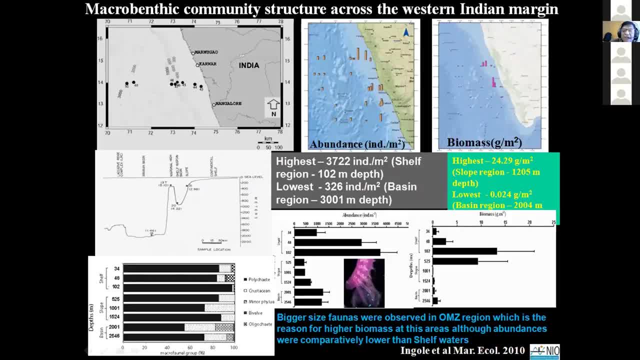 was in the self region around, you know, 100 meter water depth. lowest was in the basin around 3000 meter water depth, almost 10, 10 percent as compared to the shallower. so that's the range of abundance, what we have got it as far as the abundance. 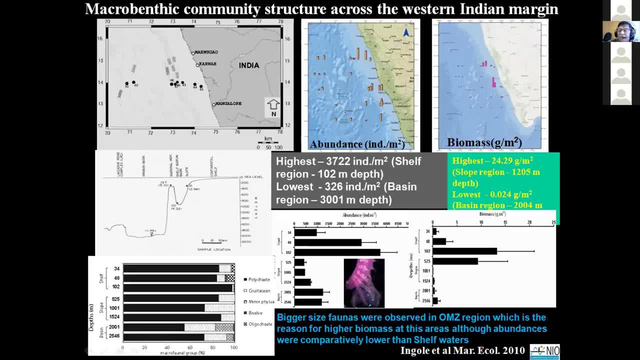 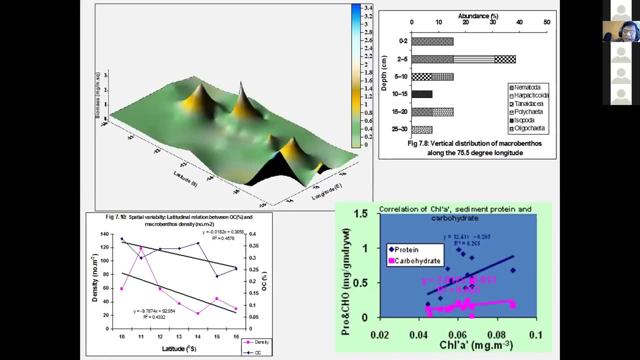 is concerned, and even the biomass is also comparable. the same way, highest in the shallower region and low in the deeper waters, As I was telling you that you know, there are, you know, very clear correlations with the food resources, although there are the patches, as I told you that. 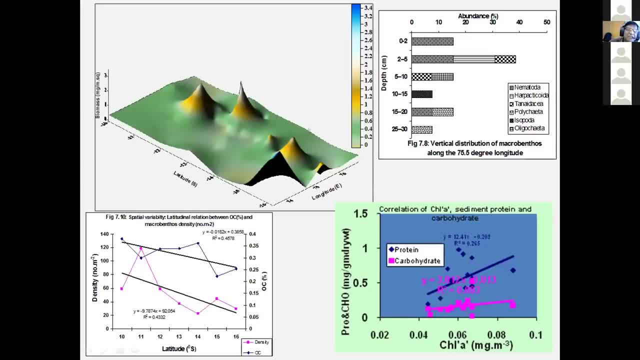 with respect to abundance and biomass in the entire basin area, if you look at it. so here you have the biomass, there are some patches that you have and this not directly related, but yes, you do have it correlation with respect to the abundance and food availability. food availability. 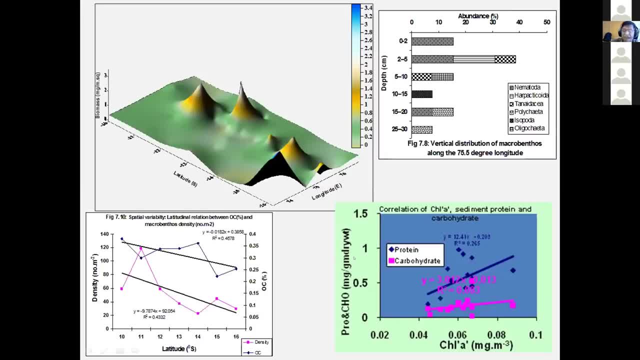 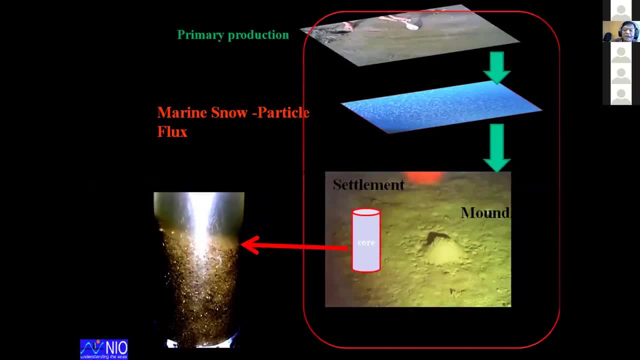 in deeper water, organic carbon, but the flux, what we get it in in the form of the marine snow or the particle plus from the surface productivity, and this is how it it works in the shallow water. we have done some, you know, seasonal experiment and we'll try to just explain how it could be. 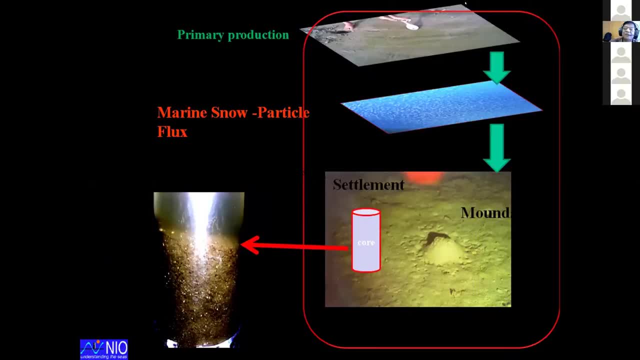 connected with the deeper water also. so we do have it: seasonal primary productivity in the surface water or the shallow water, or even in the intertidal water. very rich chlorophyll, you know production, and that's formed into the form of the blooming. what we get it, you know: phytoplankton. 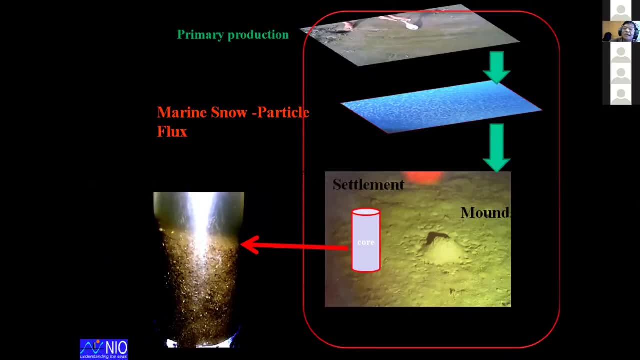 blooms sometimes, and if the blooms are consumed by the surface or, you know, phylogenetic fishery. if not, then it will the you know flux in the form of, you know sink down marine snow or in the form of, and then get deposited at the bottom and where you will get. 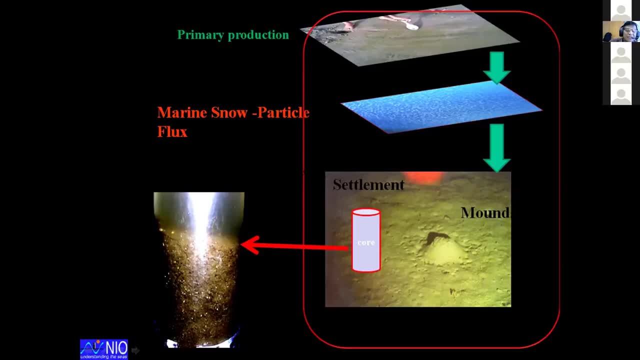 it. this is a core which is collected in the around 500- 700 meter water depth and you can see the freshly deposited green color. you know, phytoplankton are available here, so this is how it is made available for, and we did the experiment of Ratnagiri. 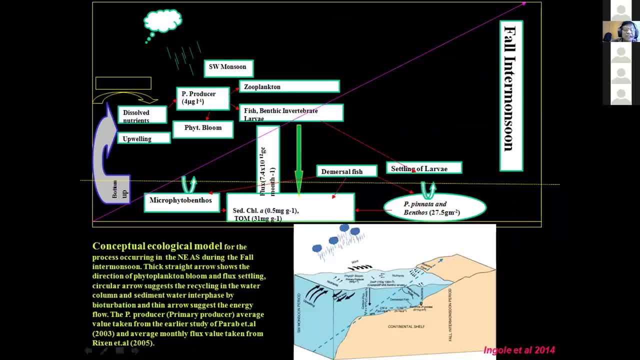 seasonal, three different cruises, we did it and three seasons, we did the sampling. we already published this data uh in 2014 and where we have seen it that we do have it. you know, uh, seasonal primary productivity: dissolved nutrient, then upwelling takes place the area, so there is a 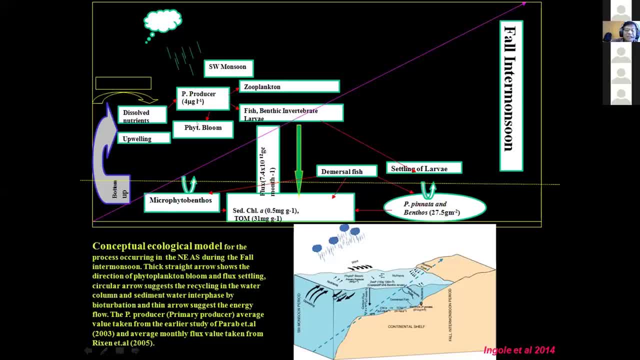 a large primary production takes place: the sink in the form of bloom, the. we have done the measurements and this is in the form of. so here is the rich micro phytoplankton, approximately benthos at the bottom, and this is a food for the. you know all other forms available in the sediment. 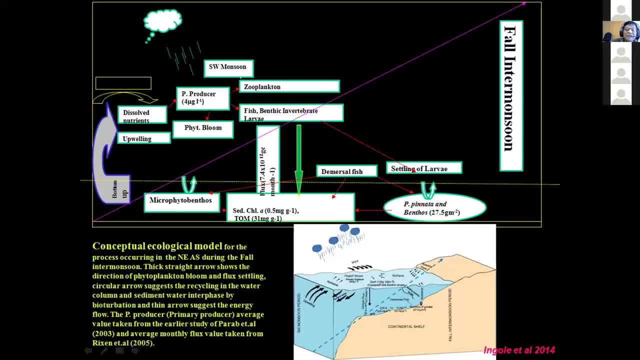 but here is a food for the zooplankton. and then the benthic larval stages are, you know, in the sediment water interface, because you're in shallow water. then you have high organic carbon present here, and that's real with the microfiber benthos. organic carbon you get in the support with the 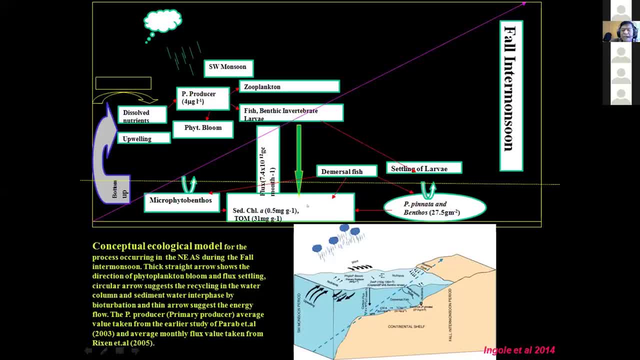 large demersal fishery and this was coincided with very clearly because your micro phytobenthos- we have high chlorophyll- contain the sediment and tom and here is the blooming of the benthic polyket, which is almost 80 percent of the all benthic biomass and abundance was the 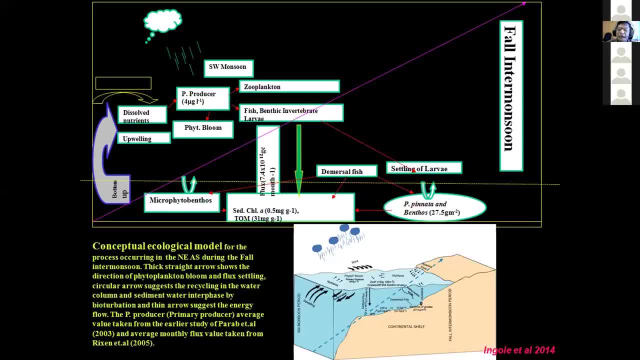 periphyllopsis pinnata, and which is a form for the demersal fish larvae in that area. so this is how it was again correlated with the demersal fishery simultaneously conducted in the area, and we concluded that the seasonal blooming, not only phytoplankton, not only support the pelagic fishery, but it will be also followed. 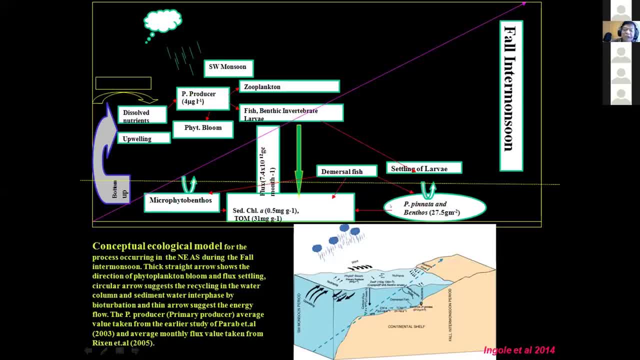 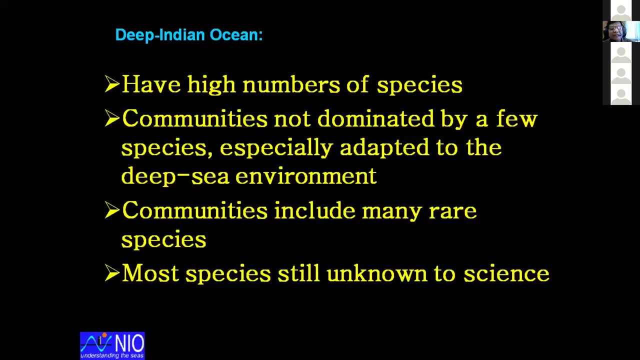 by the demersal fishery may be delayed by a month or 45 to 50 days, but it will support also the demersal fishery in the area. so this is what we, you know, reported in that one. so i'm coming to the- probably you know- last few slides. so how is the deep sea, indian ocean? 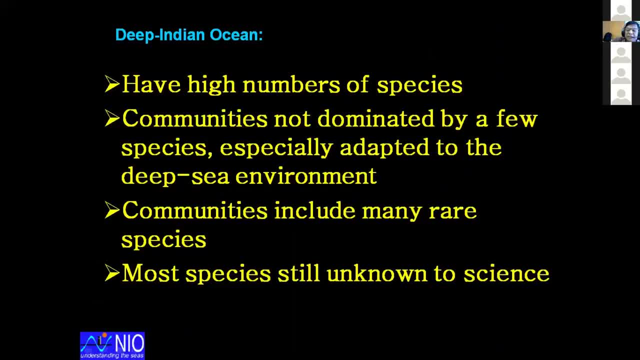 having high number of species. a community dominated by few species, as i told you, that especially adapted to the deep sea environment, community include many rare species. i'll just show you some of those things. most of the species are not known because expertise, as i told, the genus level, species level: only few species. we have been identified and we are trying to 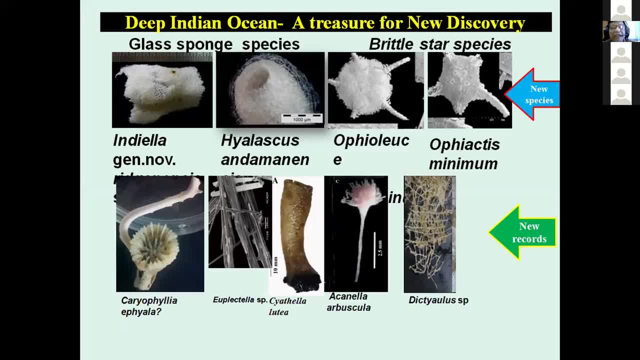 identify and we are welcome anybody is willing to, you know, put their time and expertise, for we do have the material available with us. so deep sea, indian ocean, is a treasure for the new discoveries. we already have reported couple of the new spawn species- beetle star species- and there are new. 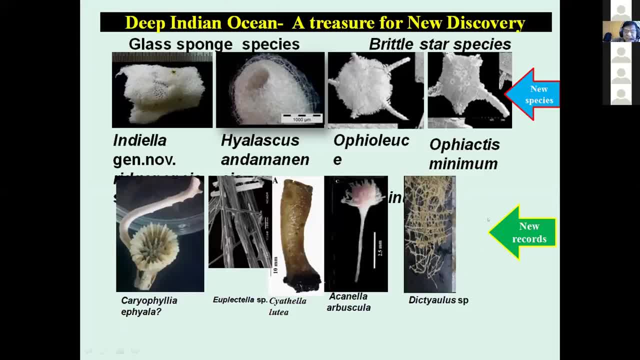 records in from this area. presently we are collecting a large number of the megabenthic species from the uh uh middle, mid, mid indian ocean, middle uh some rich areas, both from central india and southwest indian rich areas, and those are some of the forms, uh what we have recently collected i can show you. 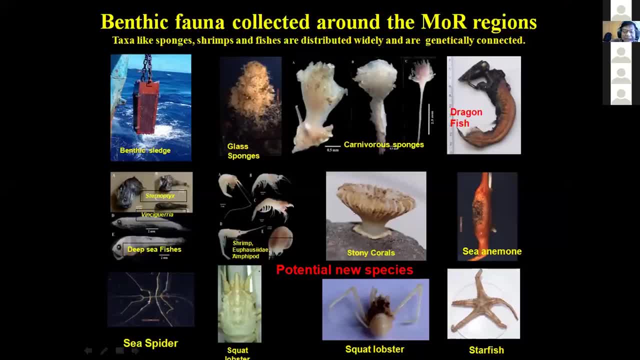 some of these are not identified. some of the identified tentatively. so we do have sponges, including the carnivorous sponges. he is a dragon fish, very rare one. you have the sea animal and and the econoderms. there are a dozen of different species not yet identified. we do have crustaceans- uh, it's got lobsters- deep sea fishes. 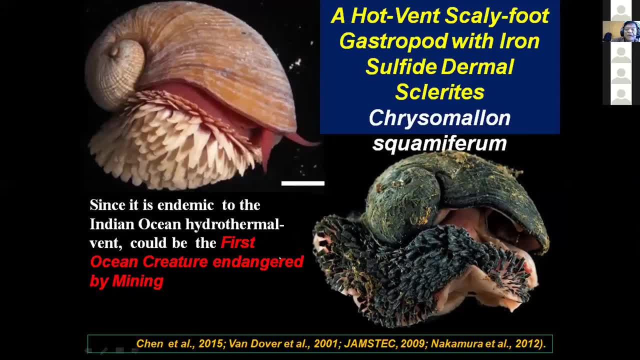 shrimps from these regions. uh, also, you know, as you know, that these are some of the area are unique, as i was just telling you that. so, uh, this is the first time it was reported from the indian ocean, this califoot gastropod, which has direct, you know, uh, association. 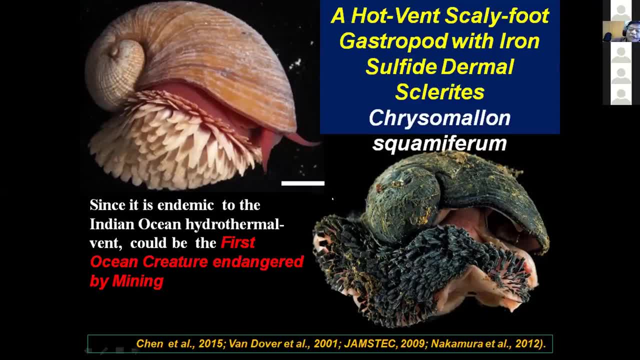 mineral deposit in the or hydrothermal sulphide deposits in along the Indian, both central and the southwest Indian reach, and this is the one species which is endemic to the Indian Ocean. so far has not been reported from other areas, but in the Indian Ocean the distribution is quite wide from. 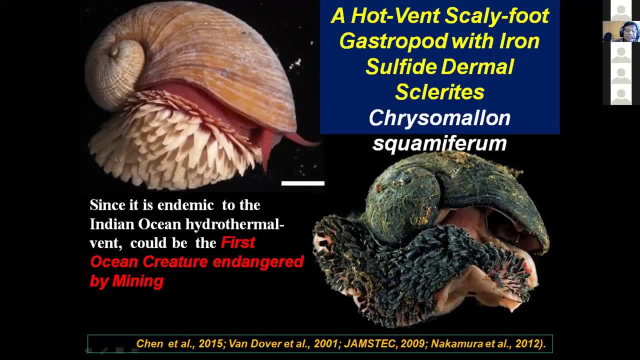 south to north, since it has direct association with the hydrothermal vent. the scientists are also speculating that if something happens in future in terms of deep sea mining, this species could be the first one which will be exposed to the commercial activity and what happens to the 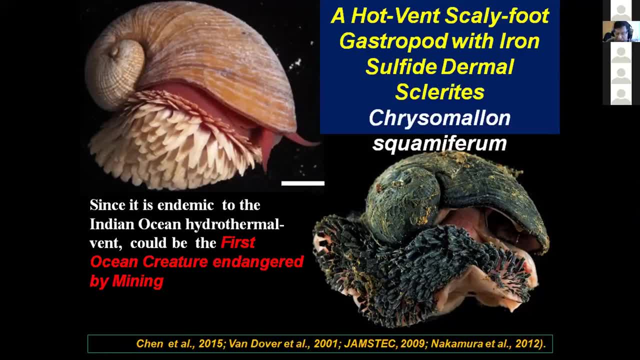 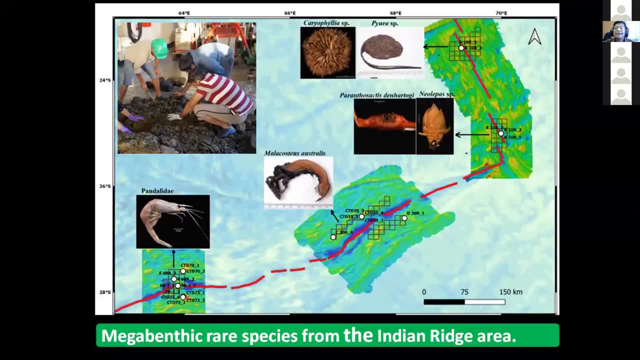 species. we don't know after that. so this is what I present, because not much information available on this except on the biology. even on ecology not much is known about this species because nearly destroyed. so distribution of some of those rare species is also quite large, early occurring species like for example hard coral or cup coral. we have got 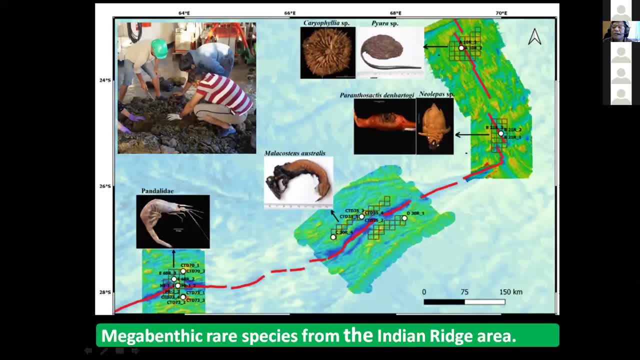 do we have to indicate deep sea? i'm telling you talking about, you know, the barnacles, goose barnacles, deep sea goose barnacles, um, see, anyone, i told you dragon fish, some of those, and then it streams and this is how they are: central indian, uh, rich, as well as the southwest indian, least from where we are collected. but they could. 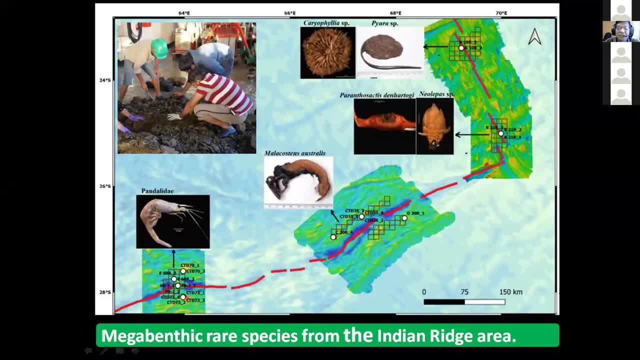 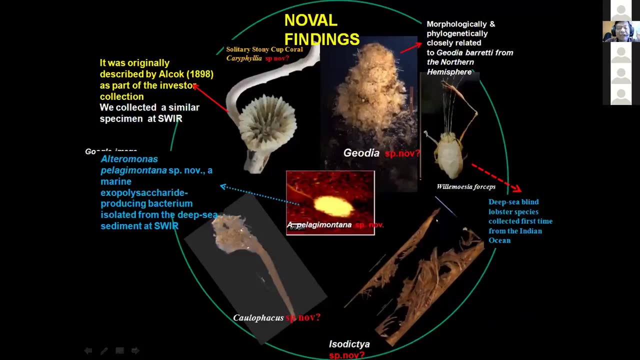 be available from available along the other areas also. that's what the genetical studies preliminary results indicate, that they are. some of them certainly, like you know, barnacles or the corals and some of the streams, like they are widely distributed, they are some novel species. as i told you, that could be the new species to the science, but some more studies are. 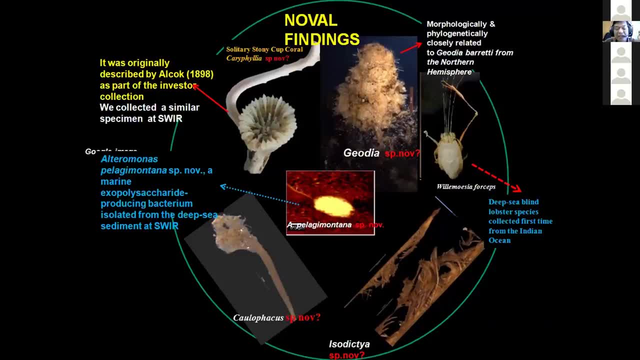 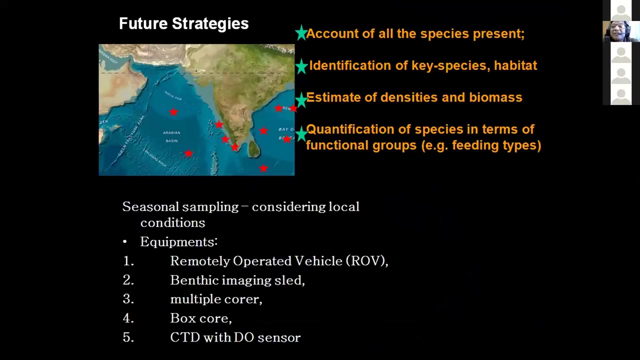 required. we are in the process of identifying, both using the traditional morphological tools as well as the molecular tools, and hopefully in couple of months we'll be able to come out with few new species in the form of publications. okay, so future strategies: what is required for such studies? that we need to do more sampling to account the species present in the 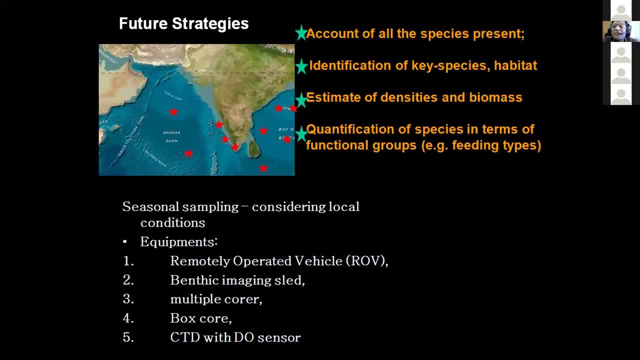 area, identify the species which are specific to the habitat, so keystone species for that particular habitat, be it the seamount, be it the self or slope, or the in the abyssal plate, because there are certain species which are dominant and they are, you know, adapted to those conditions. so we 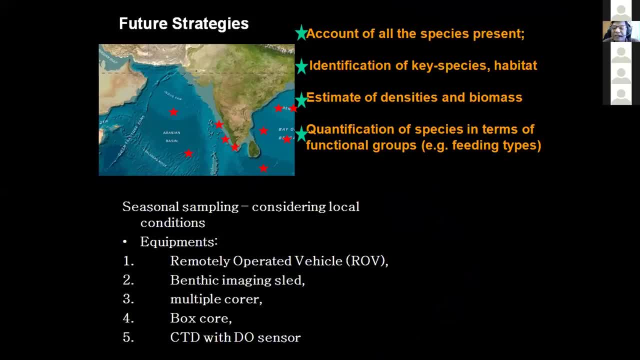 need to identify those species from those areas so that it will help. as you know, previously, you know experts was telling about the marine protected area. so if there are specific areas there are already talk about preserving some of these areas as a marine protected areas, and if we know that, 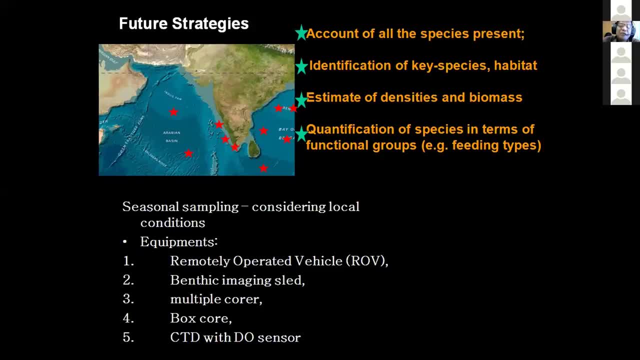 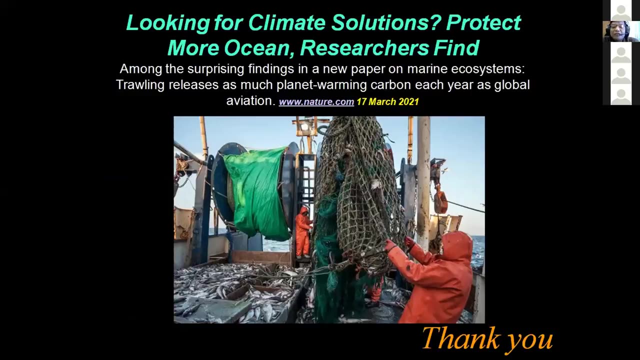 species are specific to what area, then we will be able to, you know, put some of the management practices to conserve those species effectively. okay, i have something to share, because my friend today brought to my notice that there is a new publication just came in nature, just yesterday's. 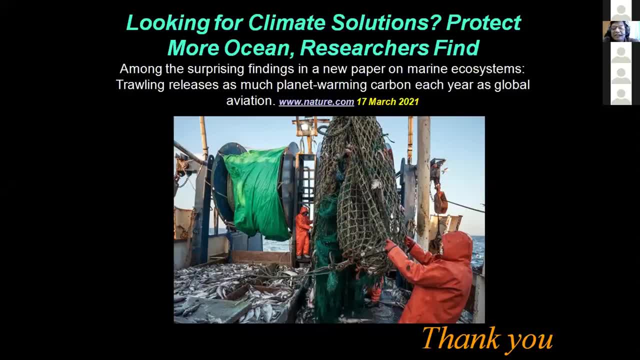 it is out and it looks like that. it is very important and pertinent to the present, my presentation, because they say that if you are looking for the climate solution, protect the marine or protect the, you need to protect the ocean and particularly protect the seabed. because what they say, that the the finding says that if you do more trawling, 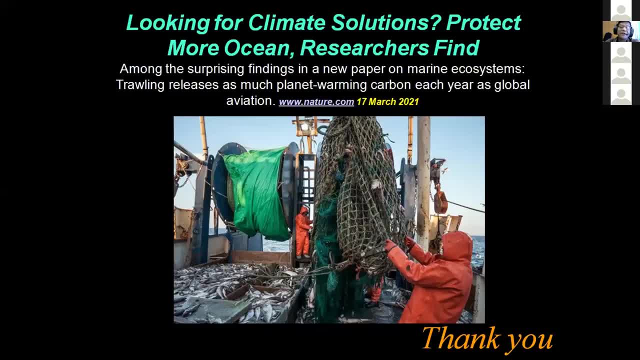 at the deep sea or the uh or the seabed, there is every chance that you are releasing more carbon, which is not a friendly for the climate. so what does it mean if there are marine protected areas or if the? if you can reduce the trawling, there will be less pressure or the effect of climate change could be. 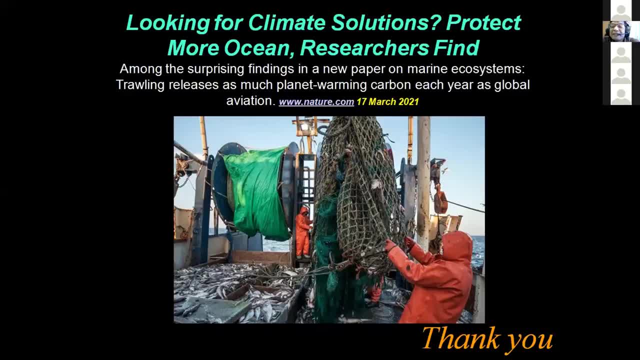 reduced. i'm not sure how it will be, but certainly the physical activity it will. if it can be controlled, it will help in preserving the biodiversity at those areas. that that is what i can, you know, say it. thank you very much for your attention.